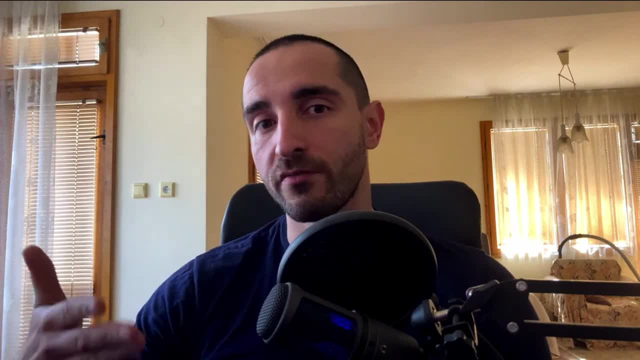 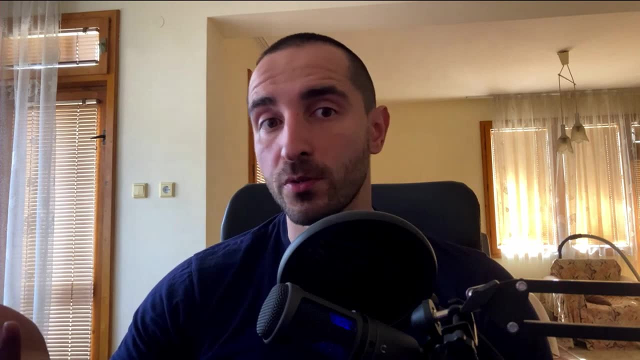 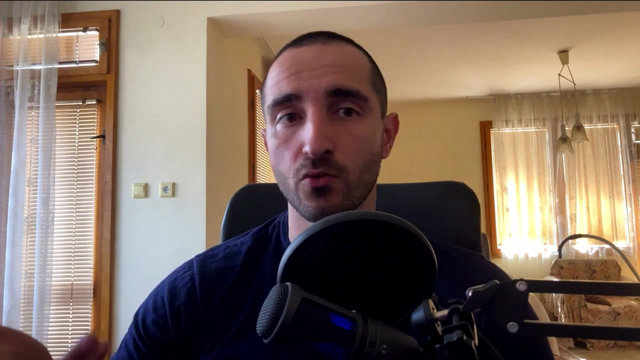 in our case, we are going to convert some multivariate data into time series sequences and the data is going to basically contain multiple features. so i'm going to show you some of the tricks that i use to convert this kind of data into sequences which we are going. 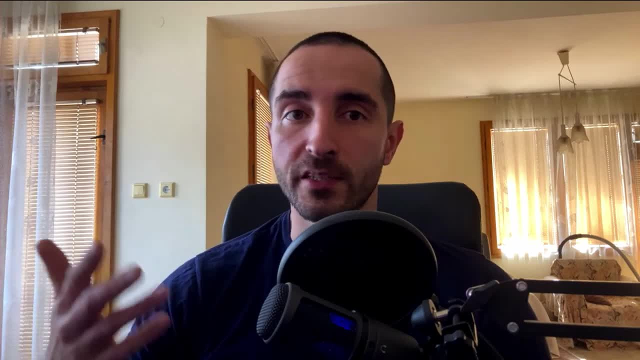 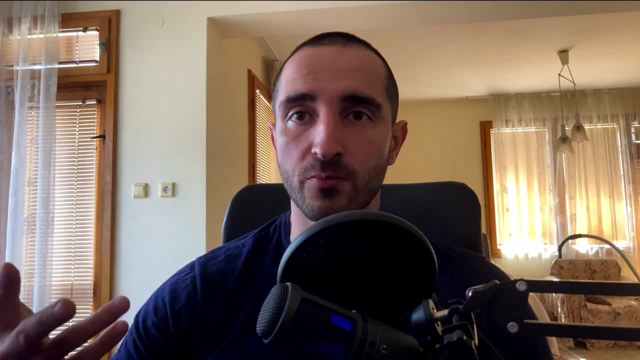 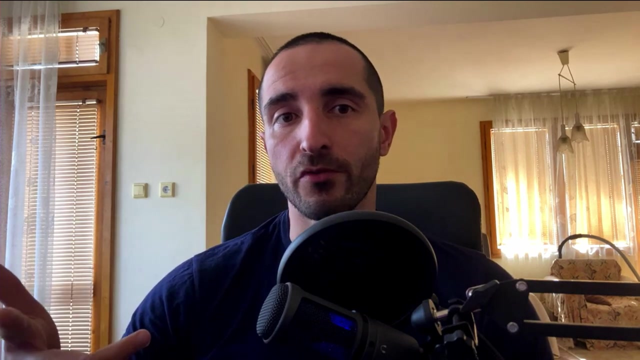 to later on convert into pytorch data sets, and i'm going to show how you can train time series data or some time series models that are based on neural networks, of course, using pytorch lightning. so stay tuned for the next couple of videos as well. let's get started and i'll show you how you can do same time series data pre-processing. 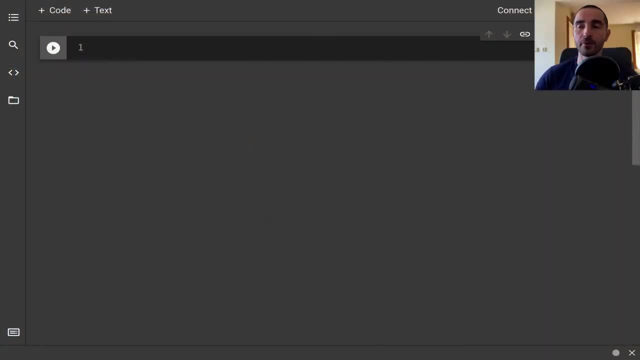 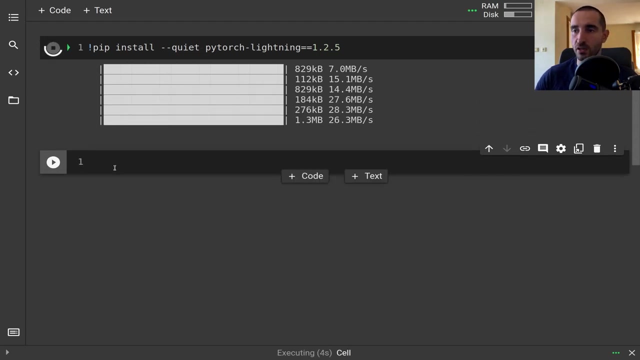 so here we have an empty notebook on google co-op, and i'm going to start by doing some library installations. i'm going to connect the notebook- we don't really need any gpu, at least for now- and i'm going to install a specific version of tqdm. 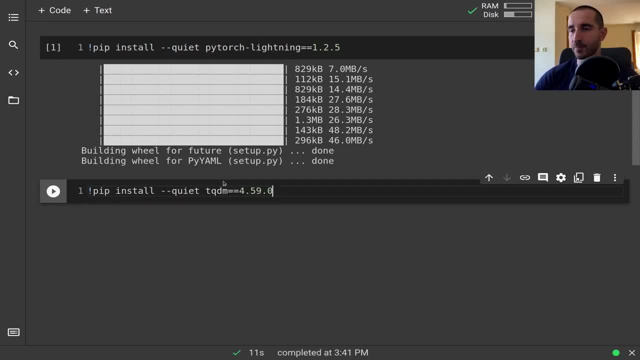 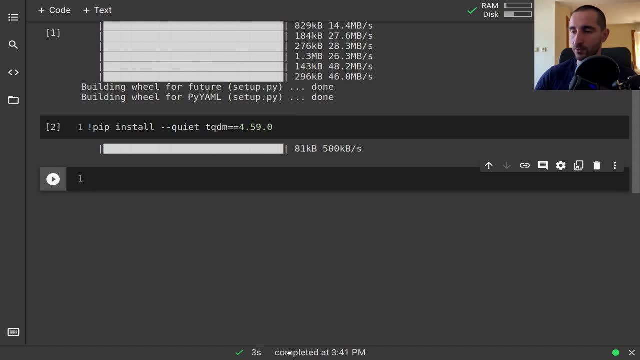 this will basically allow us to do some progress visualizations, and something cool that i've noticed about this google co-op instances, at least recently, is that we have those execution, basically statistics, and when you're doing some long running task, it tells you basically what is happening, and i'm going to show you this later on when we do. 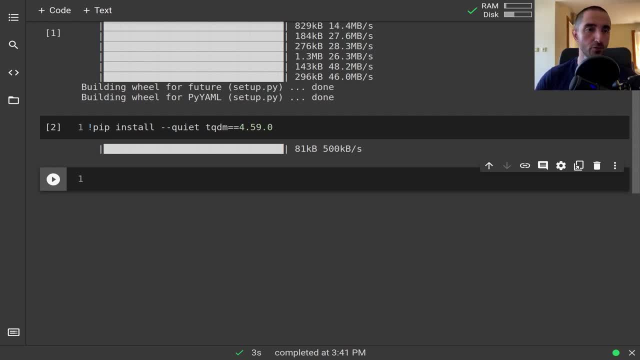 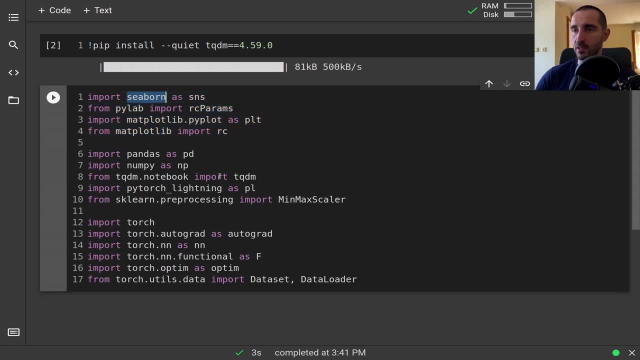 these long running tasks. next i'm going to continue with a lot of imports, actually, and here i'm importing matplotlib and seaborne for the visualizations that we are probably not going to make in this video. next i'm doing pandas in numpy. i'm going to import cqdm for the progress bars. 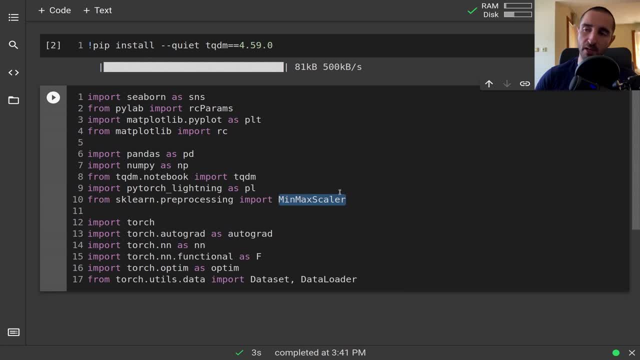 pytorch lightning, and we are going to do some min max scaling and then i'm basically importing all stuff related to pytorch and in this particular example we are not going to use many of those, but in later videos i'm just going to use some of those and i'm not going to basically 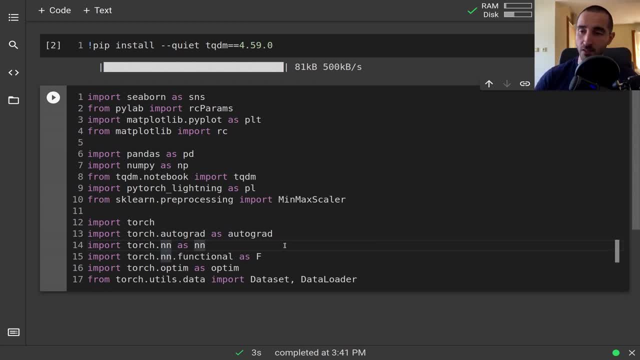 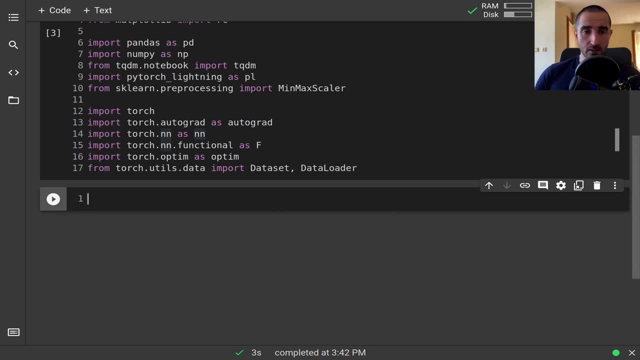 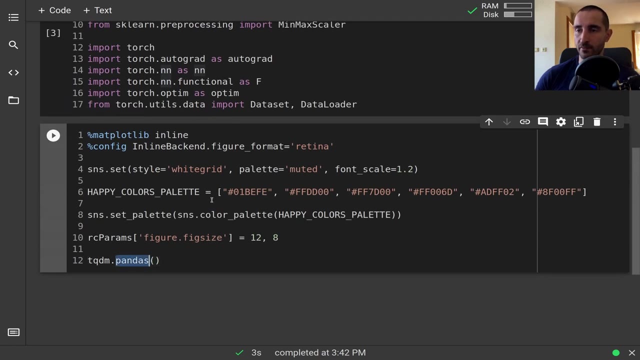 scroll up and do the imports again. so we'll do basically a bunch of imports right here and this is executing. so i'm going to also set the, the matplotlib library and the various settings for the color palettes right here and the seaborne styling, and then i'm going to import or call tqd and pandas, which will allow us to basically monkey. 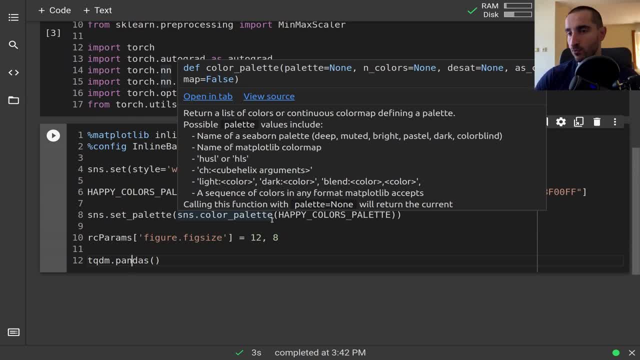 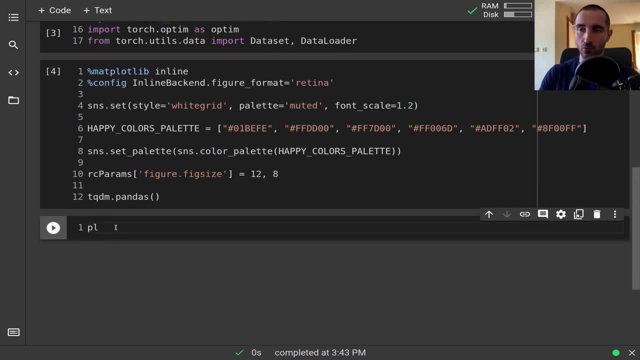 patch the apply method for pandas, which we are going to use in a couple of minutes, and finally, i'm going to call pl dot seed everything. so this is from pytorch lightning and this will basically go ahead and see everything, including some multi-processing steps that you might want to do. 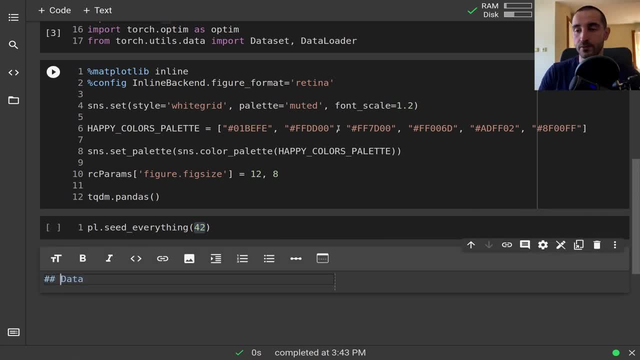 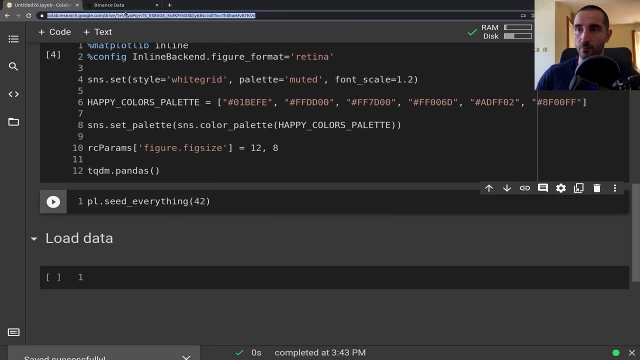 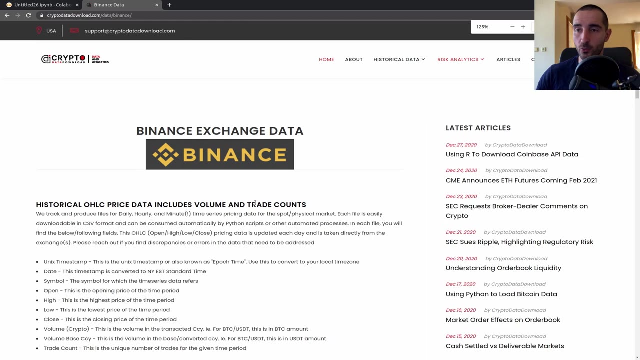 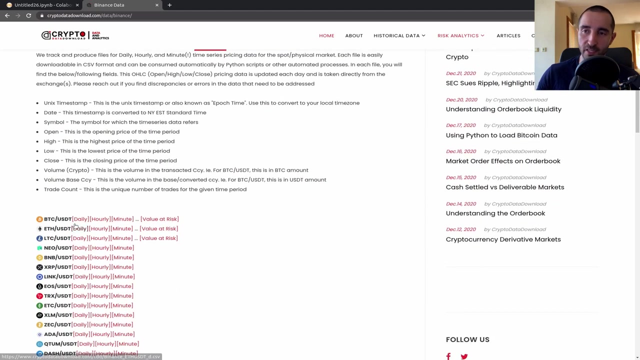 and next i'm going to what the data that we are going to use and the data itself is going to be from binance and it's provided by crypto data, downloadcom, and here we have historical data for different trading pairs. so, basically, i'm interested in this. 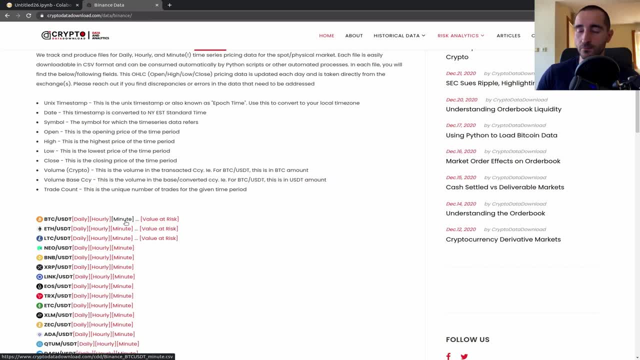 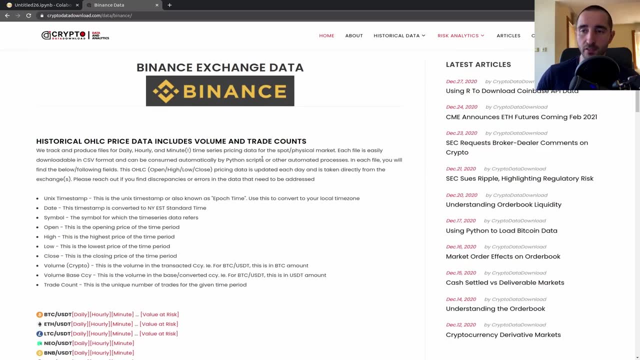 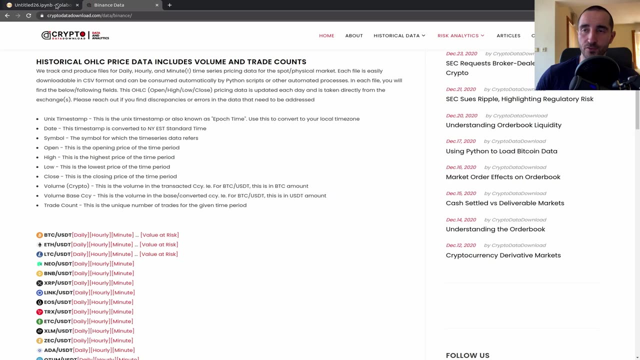 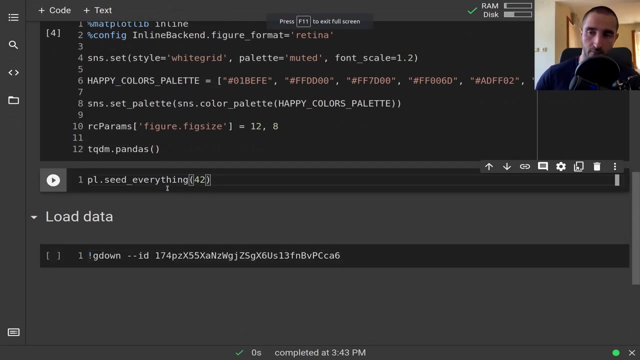 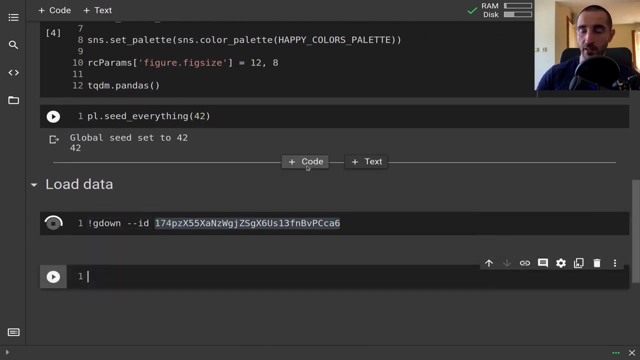 btc to us dollars, minute, minute data, and this will basically be a word of data that we are going to use and it's going to contain all those values and i'm going to show you basically what those are. i've went and used the the site to download the zip file and then i've extracted the data and from here 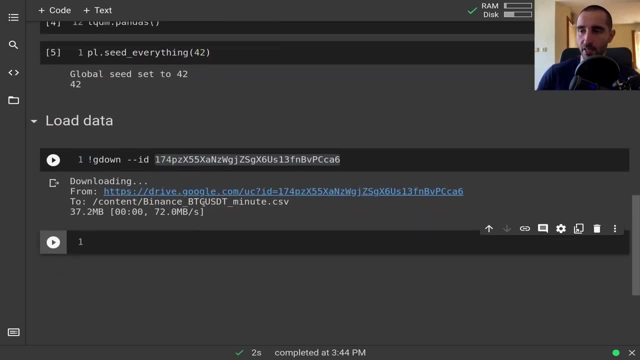 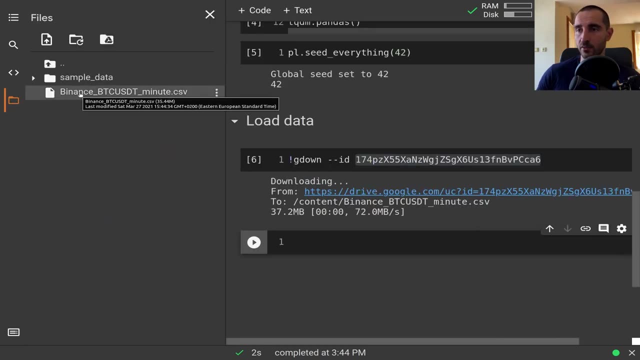 we have this binance, btc usd minute data, and it's about 32 megabytes. i believe, yeah, 35 or 36 megabytes. so next we are going to be using the btc usd data and i'm going to show you how to use it. 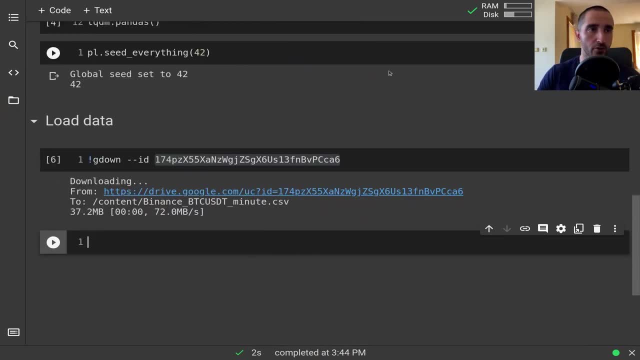 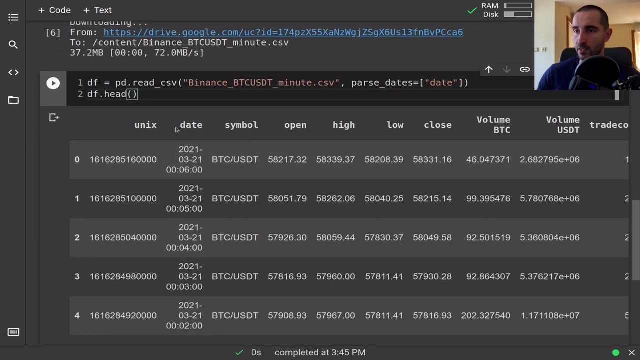 so next we are going to use pandas to read the data and this should be from the file and we get out complete here and i'm going to parse the date column and if we look at the data you can see that we have the date, the symbol which is going. 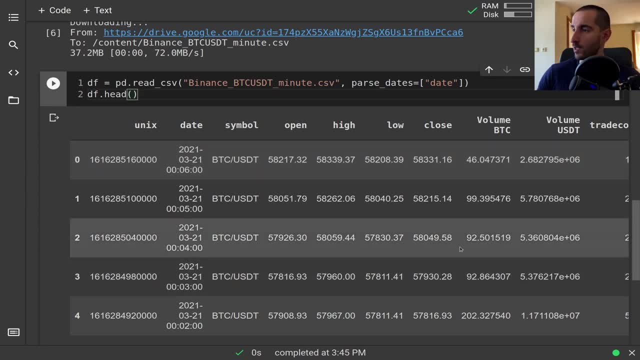 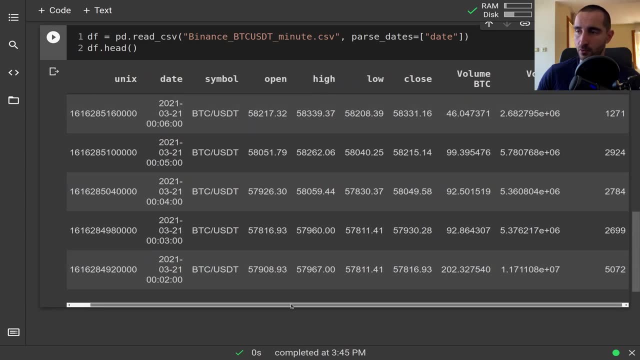 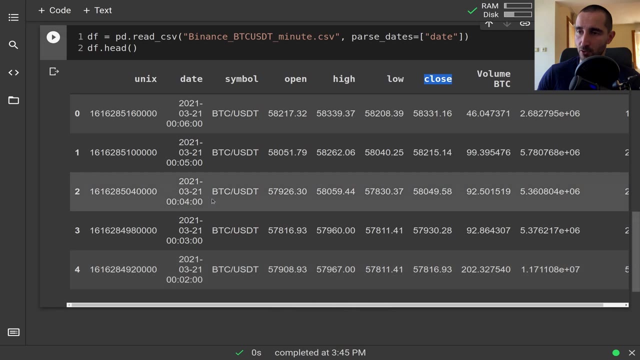 to be exclusively btc, usdt and a lot of other values which are going to be all of those stuff. so we have the opening price, the high price, the whole price, the closing price list for this minute, because this is minute by minute data and you can see that the data is. 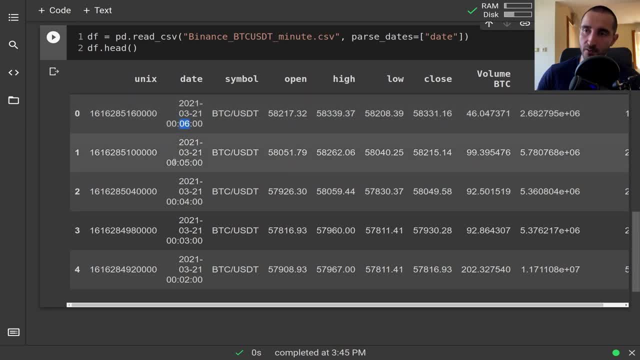 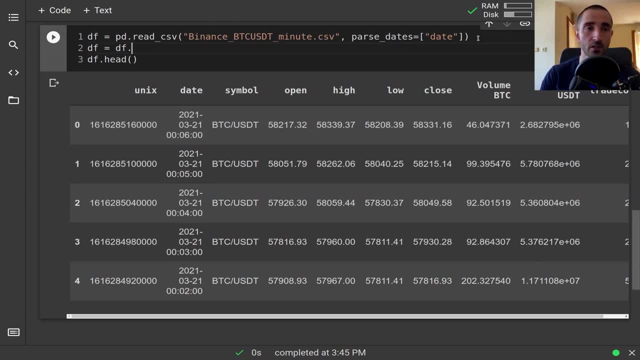 probably in reverse order, because this is the sixth minute of the hour, fifth, fourth, etc. so what i'm going to do after loading the data is sort the values by date, and then I'm going to reset the index of the data frame and right now you can see that the minute by minute data is sorted. 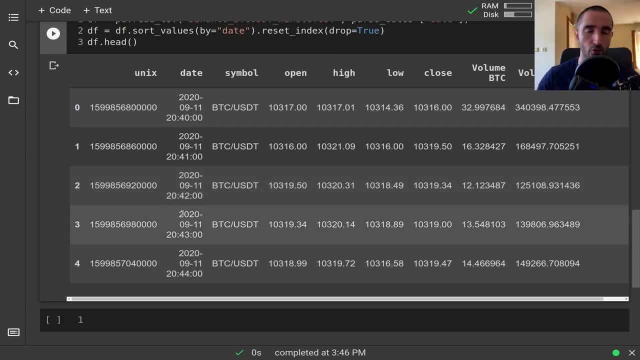 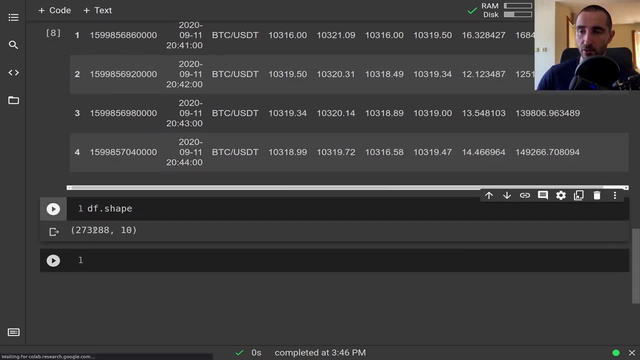 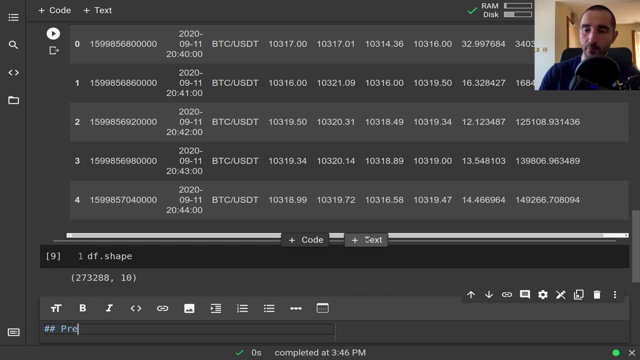 into the correct order. so this is all good, and let's check the number of rows that we have. we have roughly- uh yeah, about a quarter of a million rows, so this should be well enough data to do basically anything you want. and let's start with, let's continue with the pre-processing. 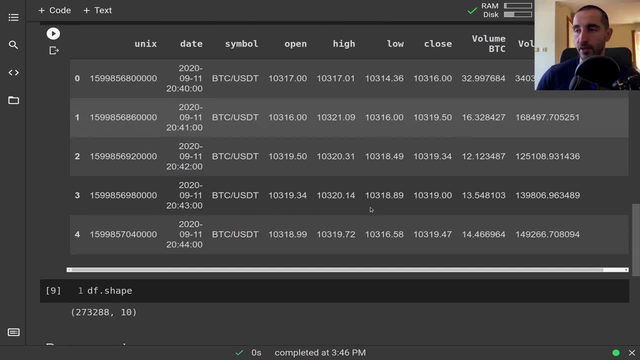 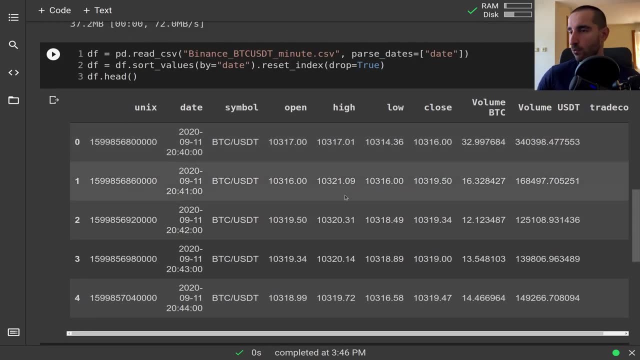 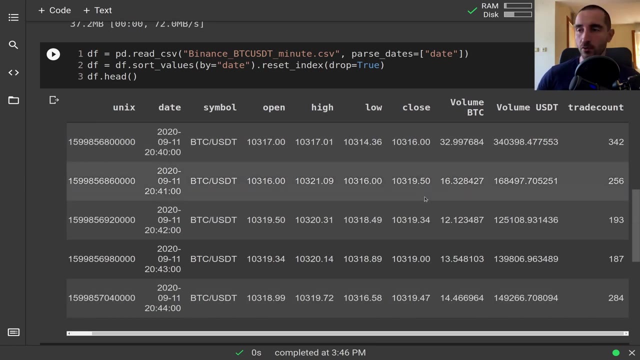 one thing that I occasionally, or very often doing is basically calculating some statistics along the current row and the next row or the previous row. so, for example, in this case we might want to have a look at what is the change from the previous closing price, for example. 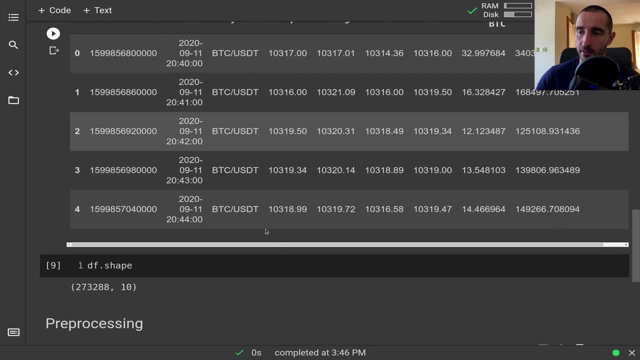 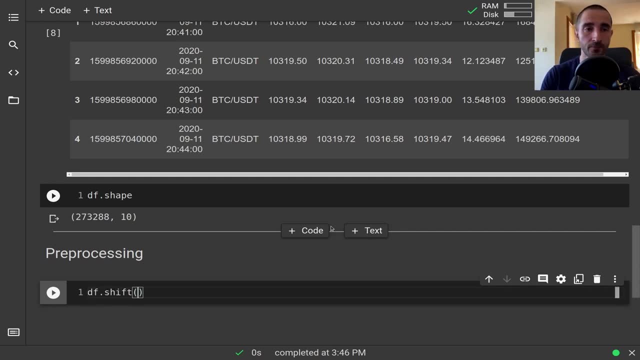 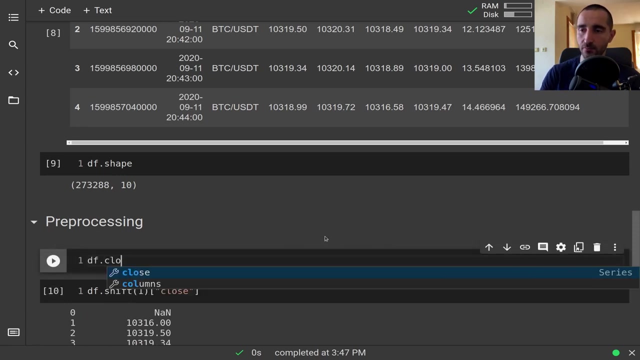 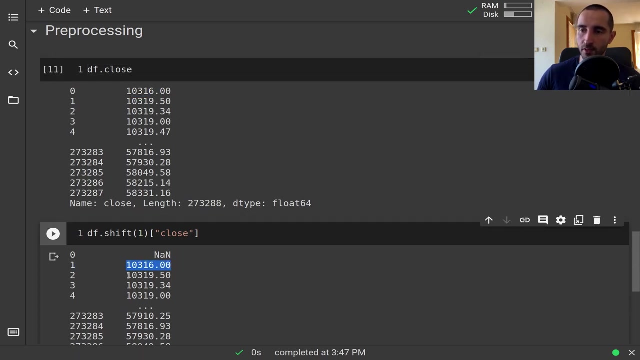 to the to the current one, and one really useful method of pandas is the shift method, and if we shift this by one position, you're going to see that the. let me just show you the close price right here. so this is the close price and this is the shifted version by one, so you can clearly see. 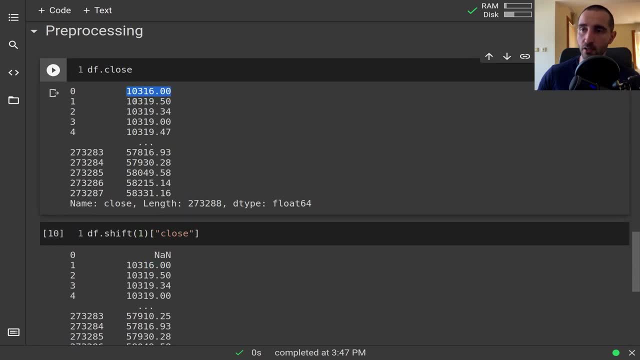 that this maps to the zeroed index right here, this maps to the second index right here, etc. etc. and and we have just a, not a number value at the zeroed index. so this is basically just shifting the rows by one, and i'm going to use this as a new value or a new column into our data frame. 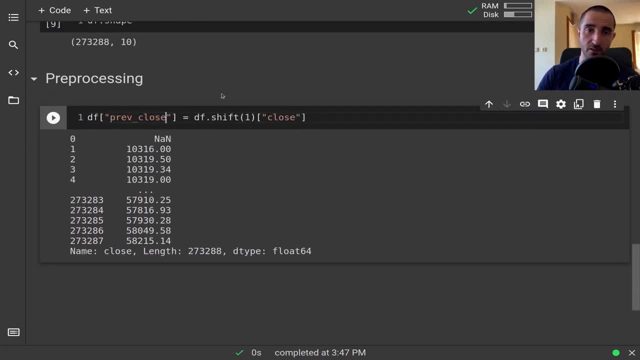 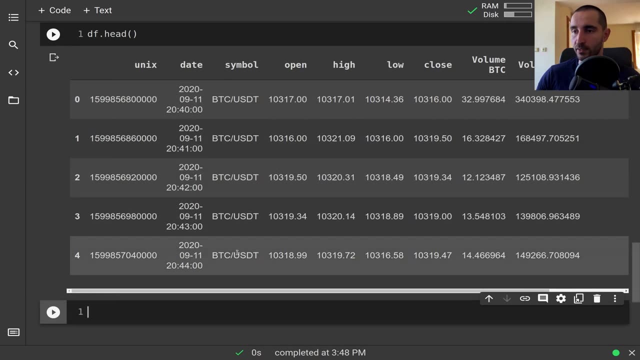 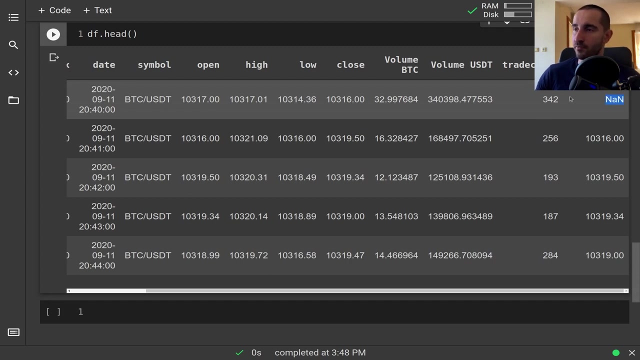 and we are going to call this previous calls, which should be descriptive enough. and if i look at the data right now, you can see that we've added this new column at the end of the data frame and the first value is not a number, which is going to be a bit of a problem, but 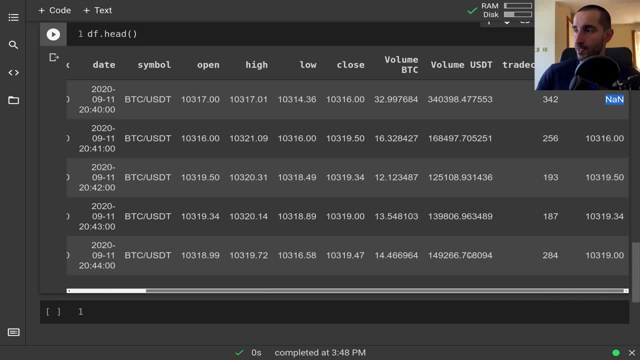 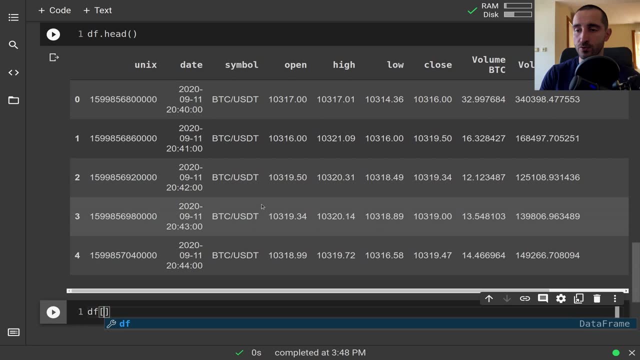 we are going to handle this right now. so we want to basically create a new column which is going to be the closing change price, and here i'm going to apply the progress program, apply function or a method which is given to us by the, the TQDM pandas library method. sorry, and 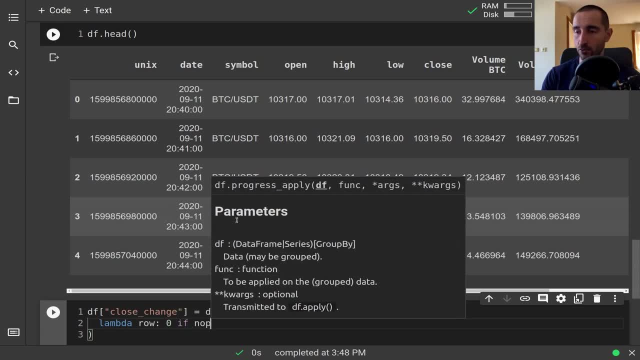 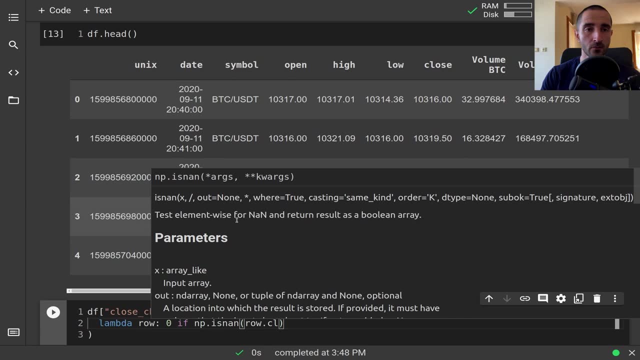 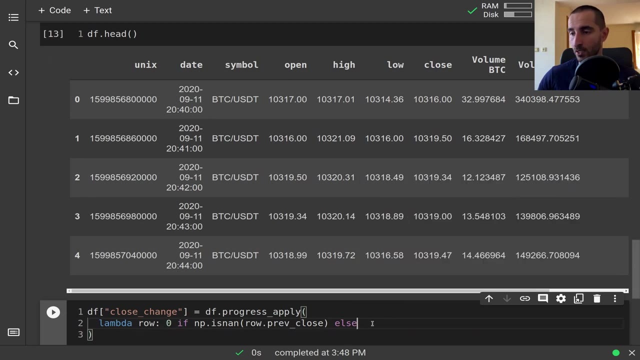 in here. I'm going to check if the current row is not a number or a none. I'm going to use the, the numpy method, for that. we are going to return a zero. else we are going to calculate the difference, or the Delta, between the current close price and the previous close price, and we are going to do 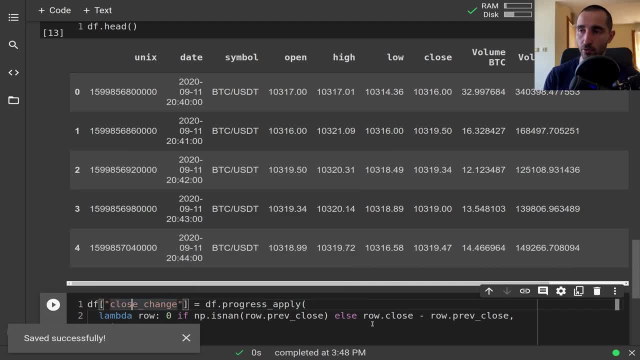 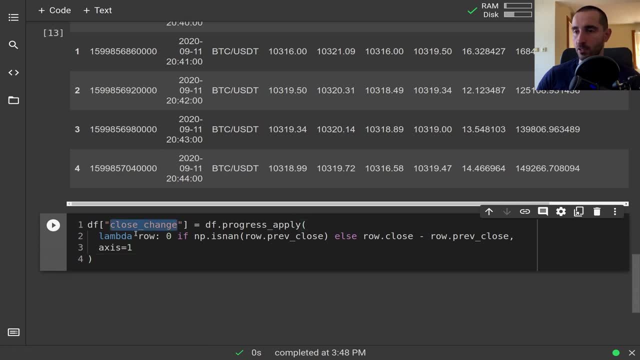 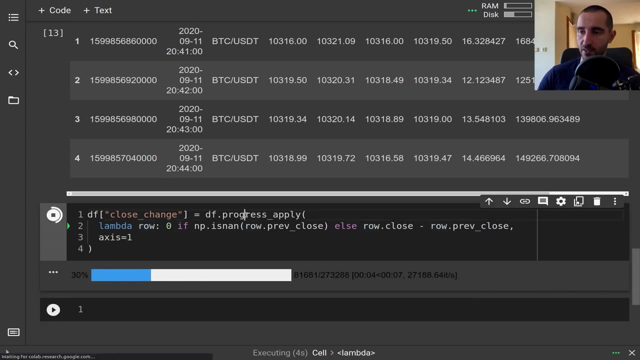 this along the first axis, which is going to apply this over- uh, the rows, basically. so this will create again another column and, as you can see, the progress apply is giving us a nice progress bar, and here is the number of seconds that we've passed during this execution, and Google Co-op is great enough to give us. 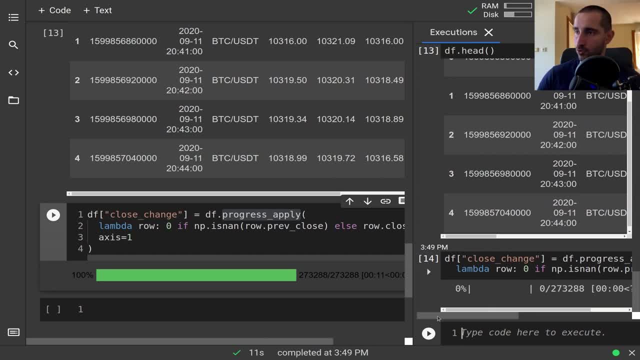 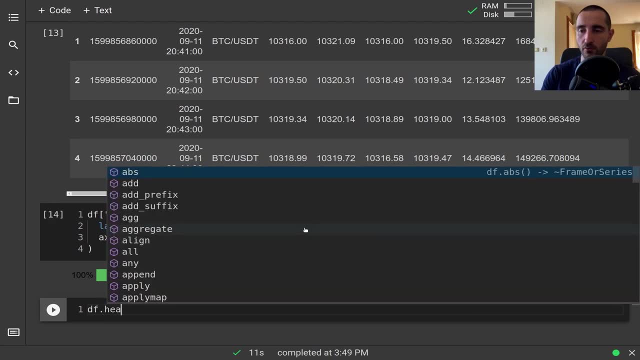 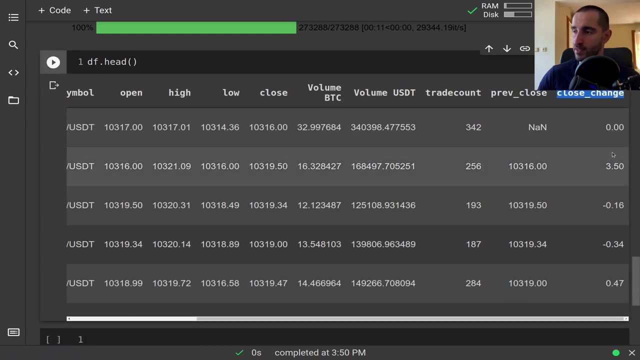 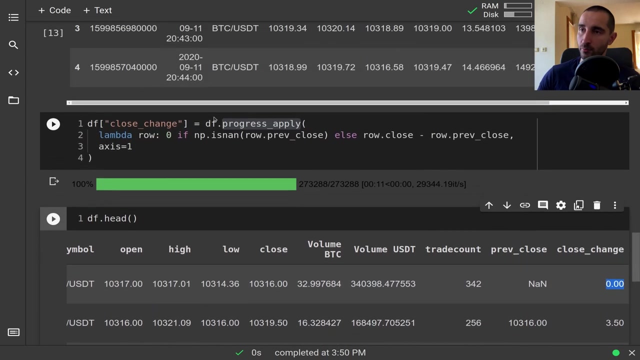 this, uh, execution summary, I guess. so this is a good feature, I believe. and then we are going to have a look at the new date frame again. we have this close change price, or the Delta, and, as you can see at the first position, or the zeroed index. we have zero because 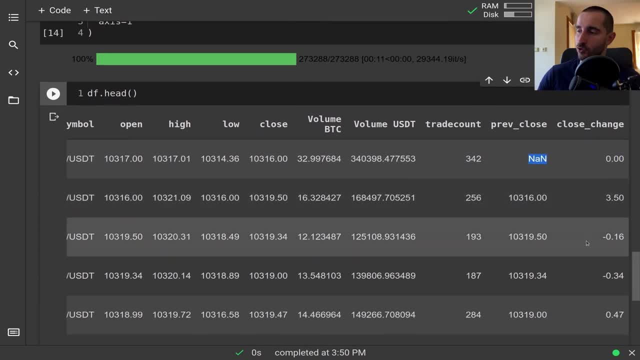 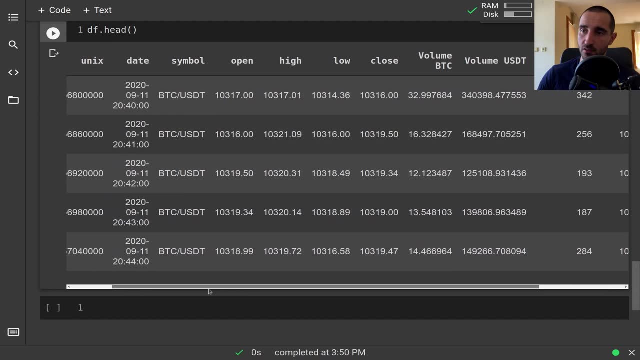 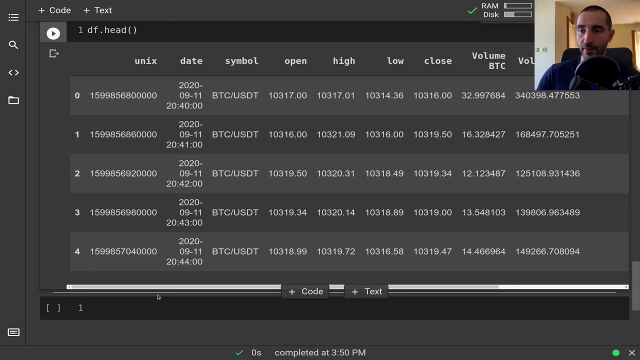 it was a non-value and after that we are just having the, the amount that the closing price has changed. I believe that this is in probably US dollars. I believe probably so. next, I'm going to convert all of this into a features data frame that we are going to use for. 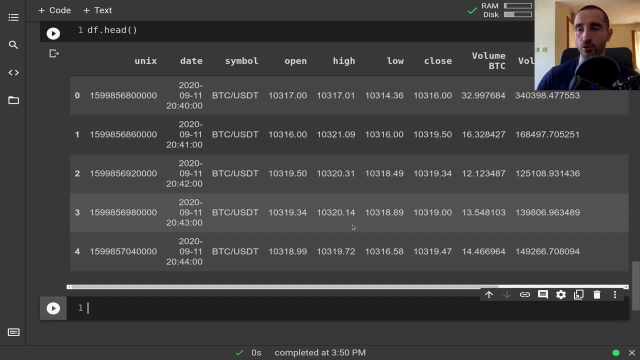 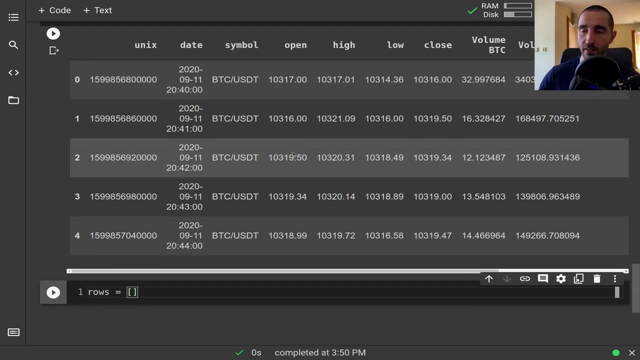 our next couple of models, that we are going to have a look at, the next couple of videos, and to do this I'm going to create rows list and in this list I'm going to basically convert of that data frame into features that we're going to use. so i'm going to iterate over the data frame. 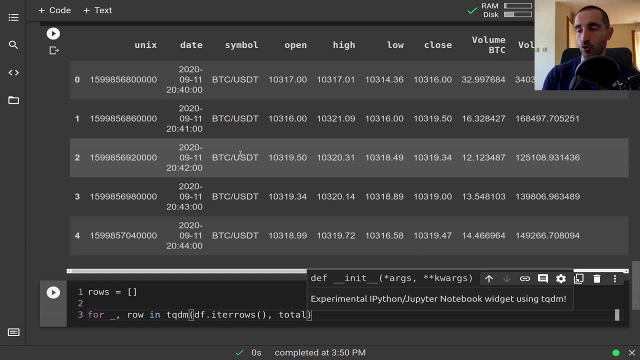 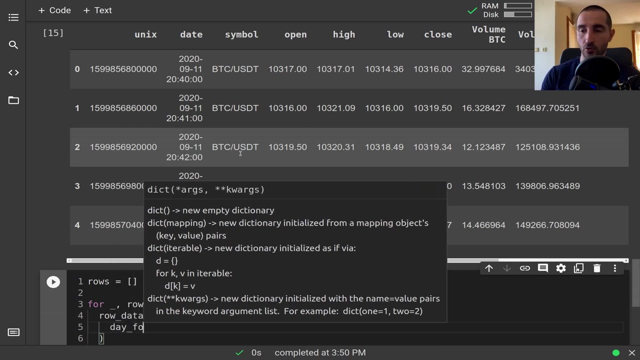 and i'm going to do that using ikgm and i'm going to pass in the number of rows that we have so it knows how many iterations we are going to do, and i'm going to create a dictionary that is going to contain the data for this row. i'm going to get the day of the week. 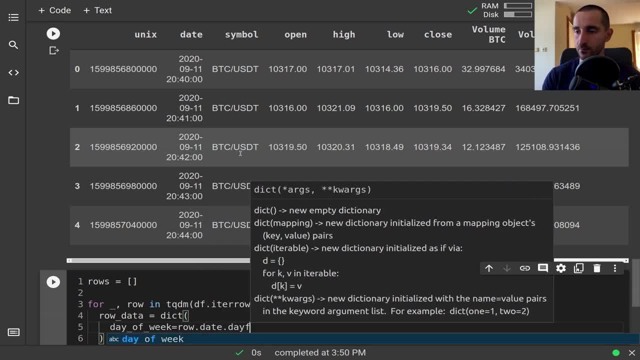 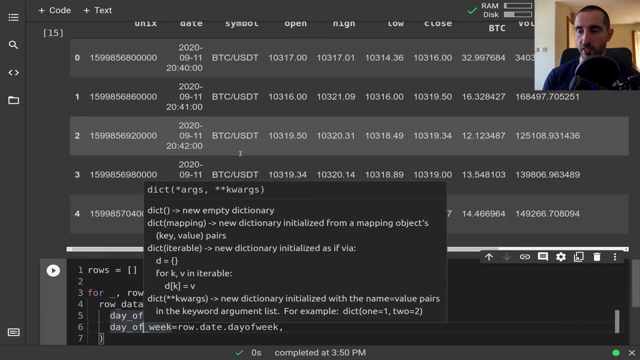 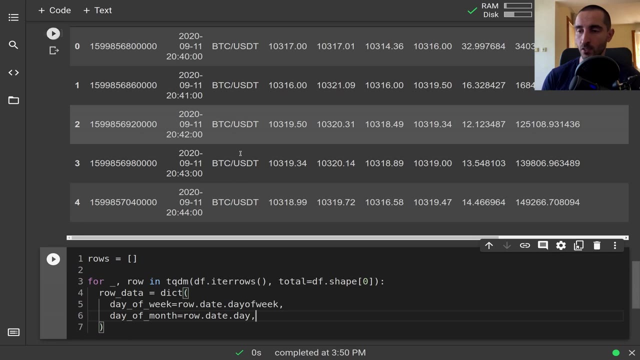 so to do that, i'm going to access the date day of week property, then i'm going to do the same thing for the day of month. this is just day. next we have the week of year, and this can be any features that you want, but i've chosen those. this is a way to basically encode the date. 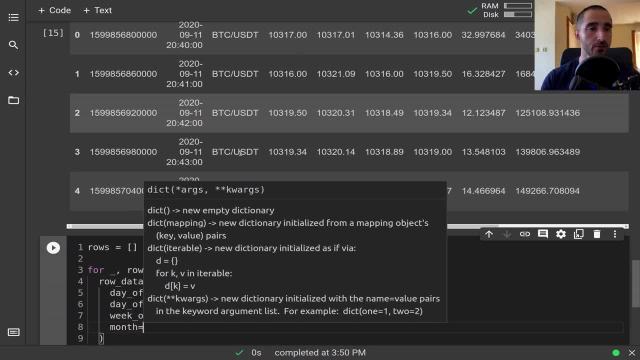 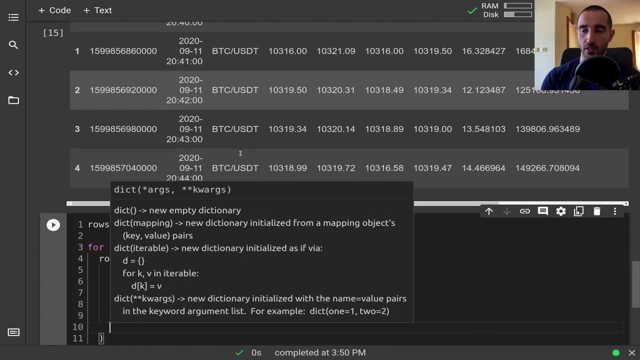 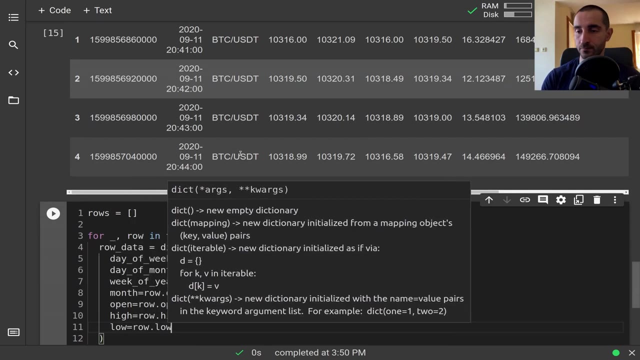 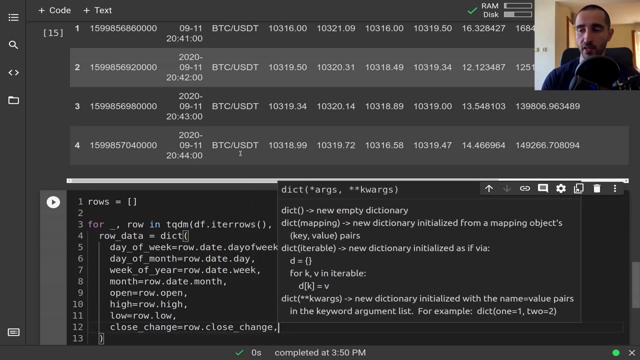 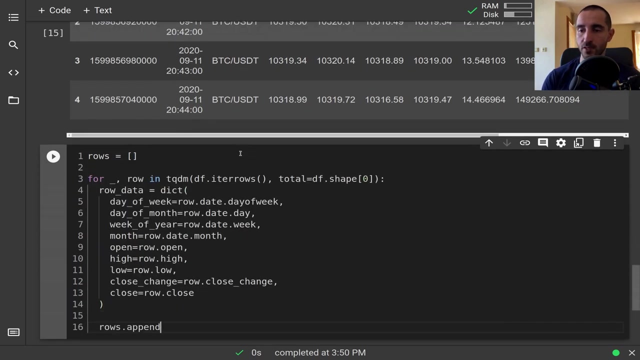 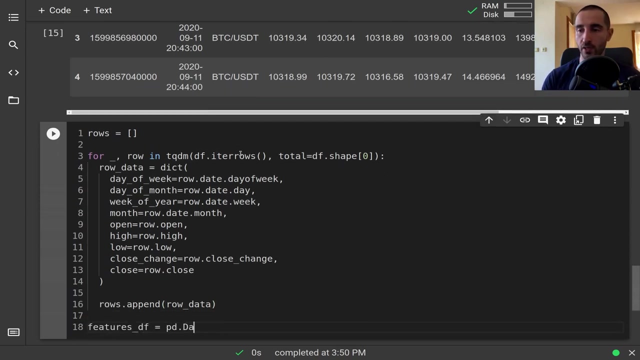 next, we have the month and the opening price, the, the high price, the low price, the close change, which is going to be the newly created feature by us- and then, finally, the closing price, and i'm going to append this to the rows and i'm going to convert all of it into a data frame. 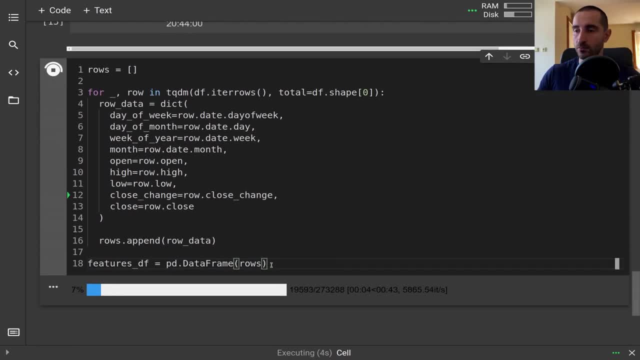 so here is again tikkm, and one interesting thing about the google co-op thing is that it's jumping all around, probably telling us where the current execution point is. i don't know, but it's doing something all right. so after this is complete, i'm going to 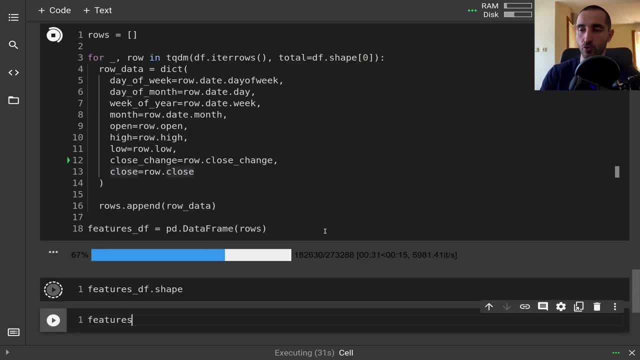 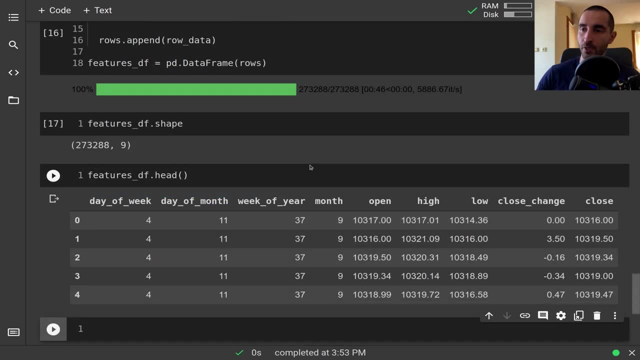 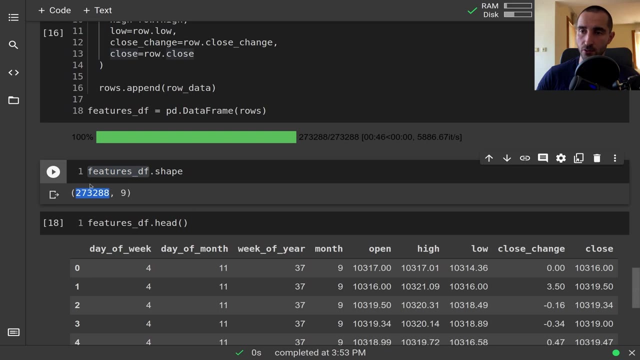 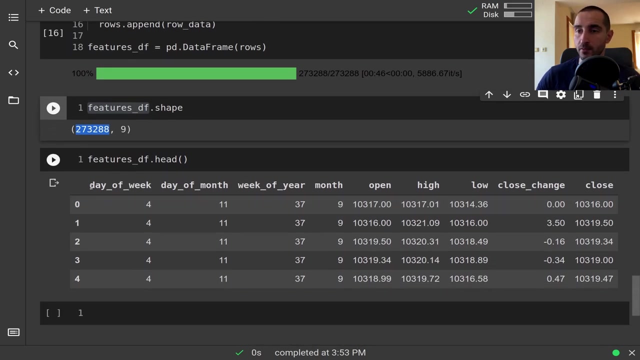 just check the shape of it and then i'm going to have a look. the data frame itself. now that the feature creation is complete, we have this newly created data frame and it has all the same number of rows that we had before. but again, we are just doing. 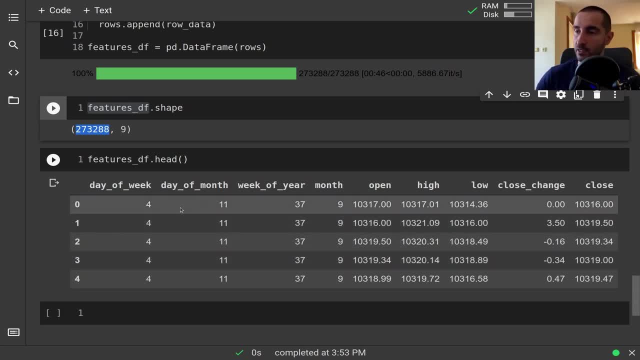 some feature engineering, if you will, and in here we have the new numbers extracted from the original data. next, we are going to make the split between training data and test data, and in this case I want to have 90% of the data for training, and I'm going to do that by calculating about 90%. 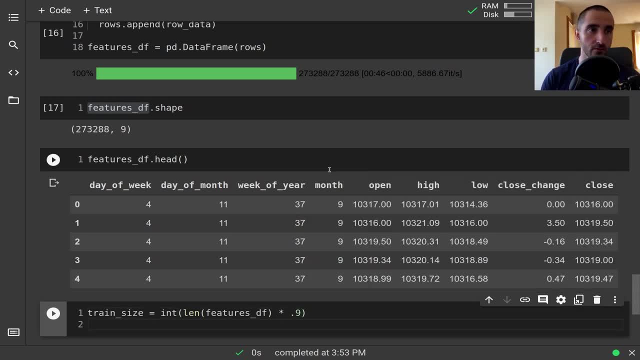 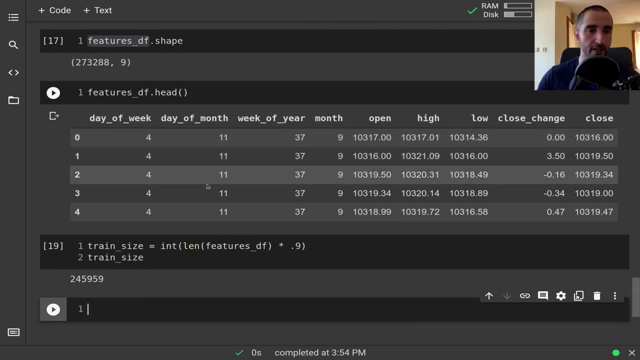 of the features, the number of rows that we have, and this will calculate the come out to this number. next, we are going to split the data frame based on this index. we are going to create those two data frames and I'm going to use the features data frame. 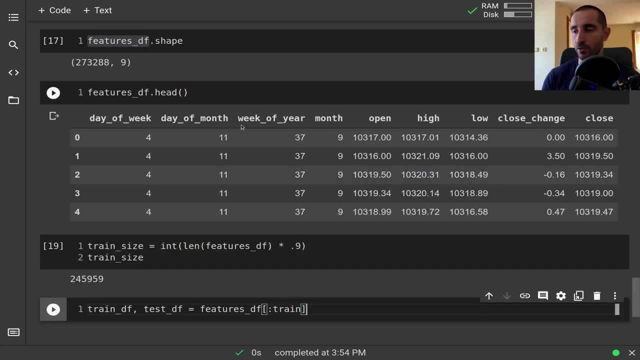 and get all of the examples before the train and then I'm going to take all the examples- sorry, the train size- after this and I'm going to take the few of the 이야 from the form page, that is, that is folding out one whole. we are going to stamp these books, so now we get to see the difference between the now actually. 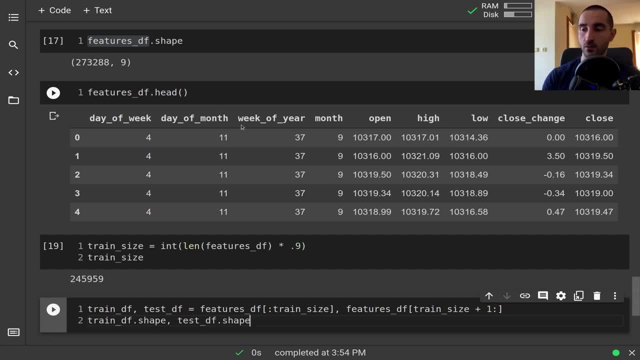 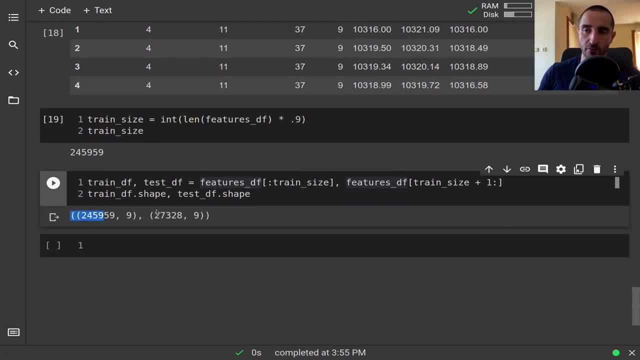 the behavior for angel data is the same for transformation, just like any typical introduction, when the object on the model is Boolean and the origin of the element was Find Inventor term and we can see that we actually use understood a lot of this in the syntax. 001744064117, Yamaha. for each data frame, we are able to add one just to make sure that an old data is leading between the training and test data. it is leaking between the training and test data, same numbers that we have for training and testing. as you can see, we have let them and, as you can see, we got the numbers that we have for each data frame, which is good, as usual. 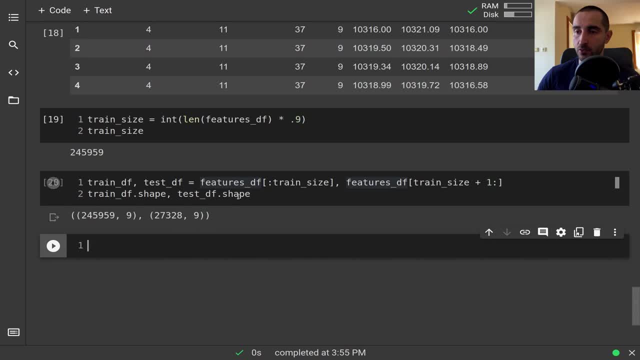 good, and next we are going to do some transformation of the data, and the transformation that we're going to do is basically a min max scaler or scale the data. scaling the data allows us to probably get faster convergence when training with stochastic gradient descent and and when using probably deep neural net models, for example lstms or grus or one. 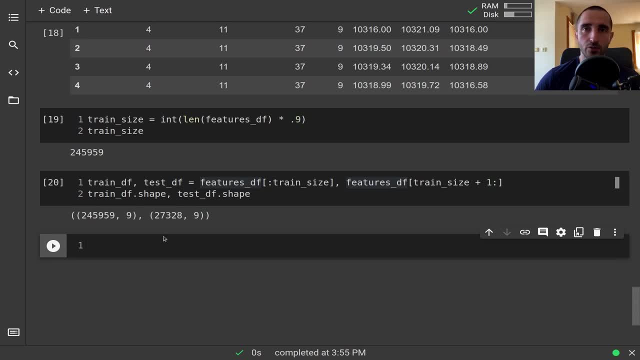 one confs, or maybe you, if you are kind of on the cutting edge, using transformers from for time series data. in all those cases we are basically training with stochastic gradient descent. so scaling the features and the labels helps us to get faster convergence and we're going to do that in the next video. 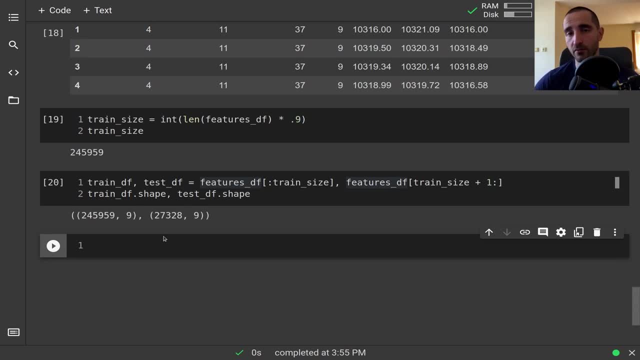 get a bit of better results, faster convergence and probably is going to fight against the exploding or vanishing gradient problems that you might have. so one really easy way to do that is to use this sk1 min max scaler, and in here i'm going to specify the range minus one to one. so this will be the range that 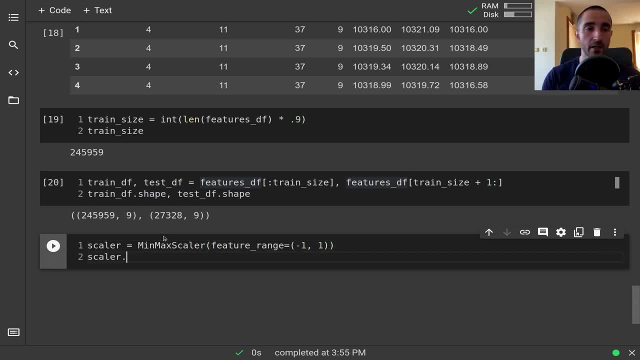 all of the features are going to be going to be the range that all of the features are going to be going to be scaled to. and then i want the scaler to fit only the training data, and this is very important because we don't want to leak any of the test data that we have thus far into the scaler. 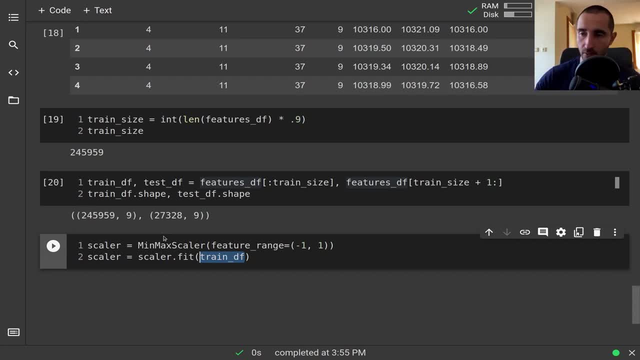 we want to scale the the data using only the mean values and the standard deviations of the training data that we have. so the test data is going to be the training data that we have. so the test data is going to be basically going to be basically just for testing, and we did the same thing here with the split. 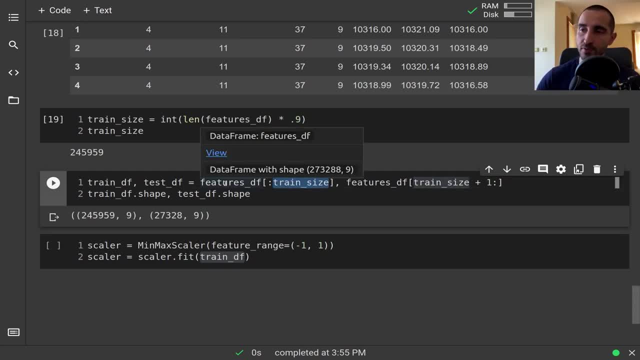 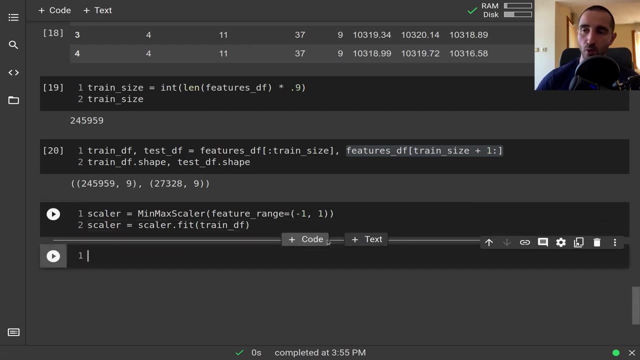 we first got the first any examples, and then the later on, as the time gets on and on. we are reserving this data for testing. so this is really important because you don't want to leak any data from the train, uh, from the test data, before evaluating it. next, i'm going to apply the transformation of the scalar. 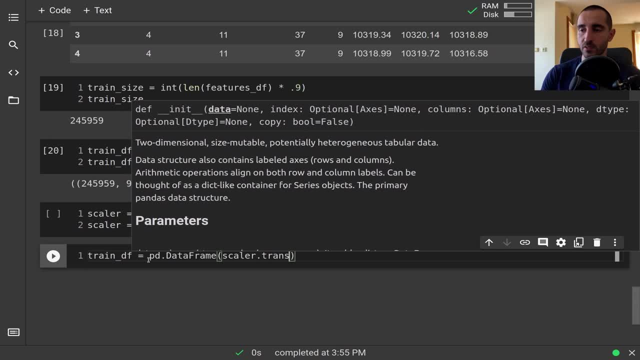 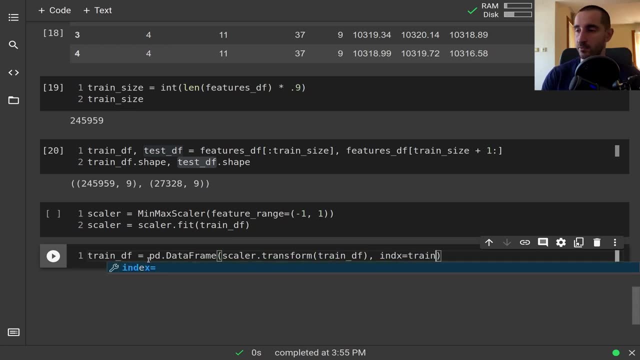 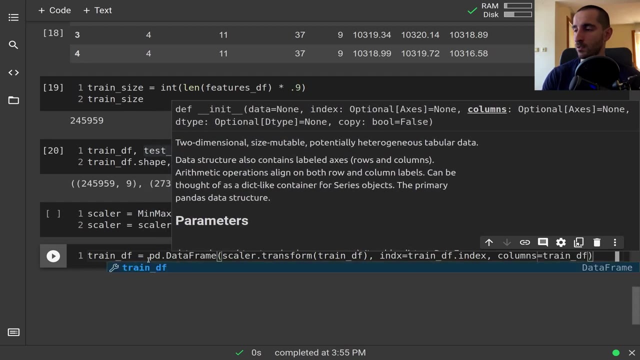 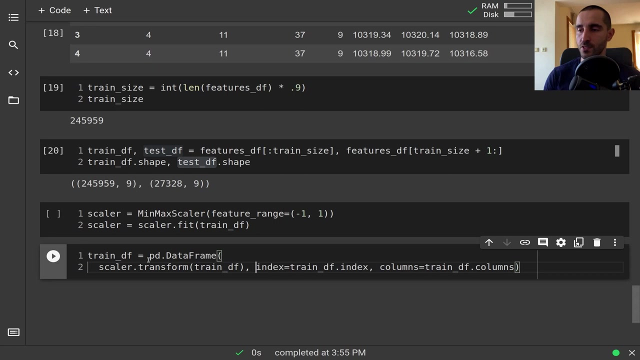 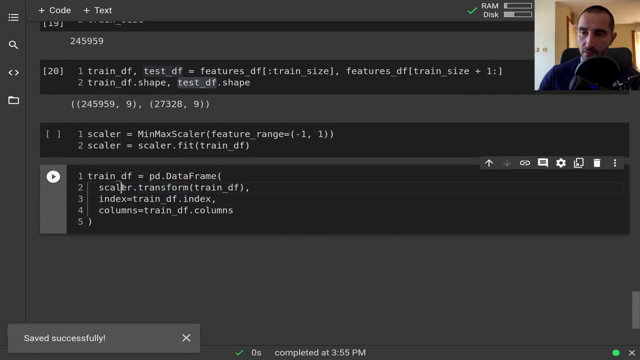 and i'm going to call the scalar transform method on the training date frame and i'm going to pass the train gf index and the columns. so, yeah, this is getting ugly, so i'm going to re do this. so why we're doing all this? uh, basically, if you just pass in the scalar transform df, let me. 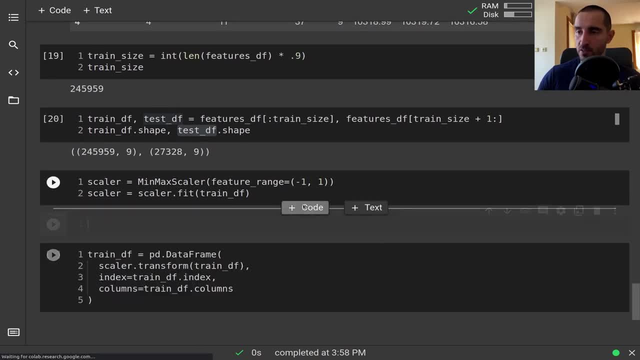 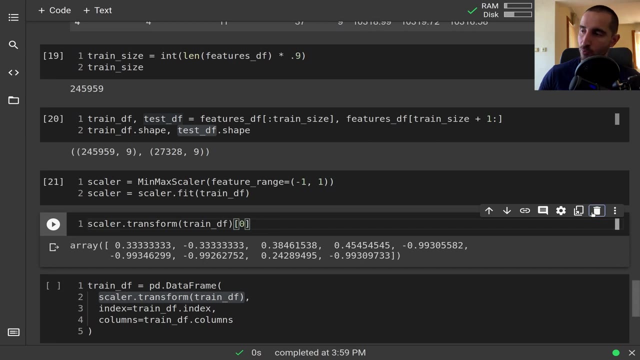 actually execute this and i'll show you. if you pass in the scalar transform brain df and look at the first row, you will see that this is no longer a data frame and just to preserve the data frame itself, we are going to do the transformation, but we are going to basically create. 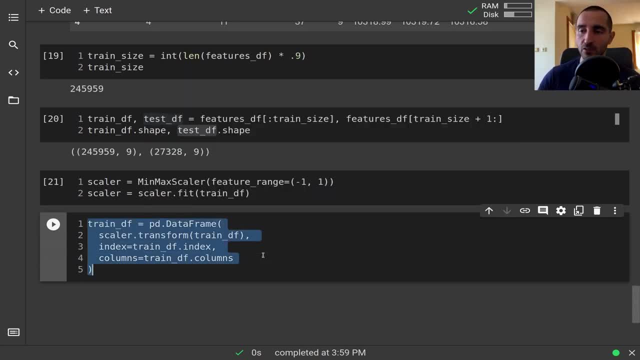 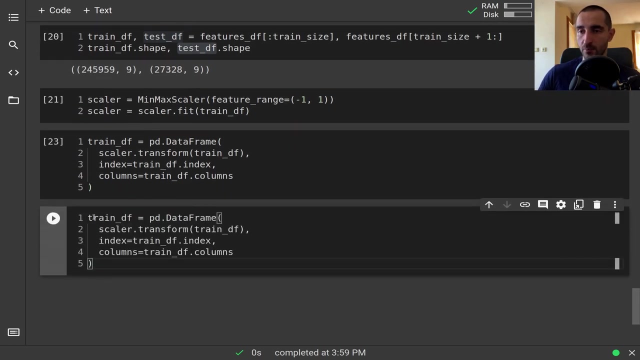 a new data frame. that is the same data frame that we had before, but in here we are going to pass in the index and the columns and, of course, the transformed values, which are going to be this numpy array. so i'm going to do the same thing for the test. 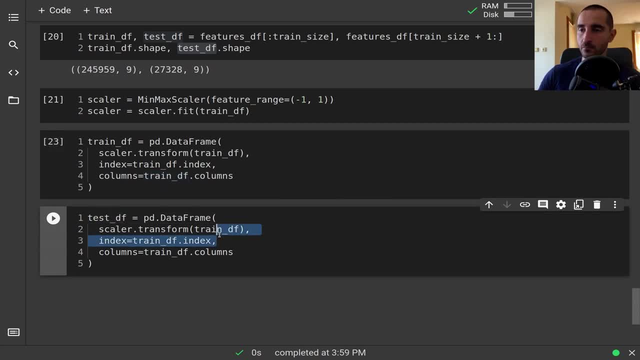 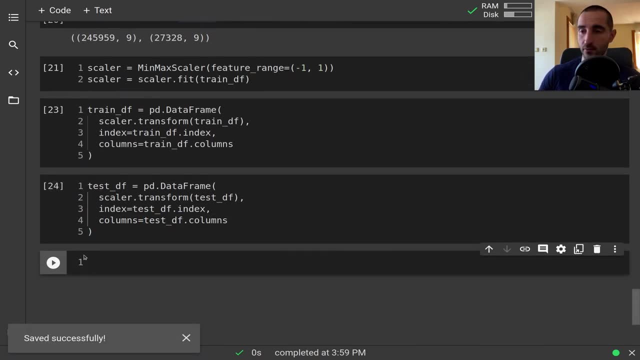 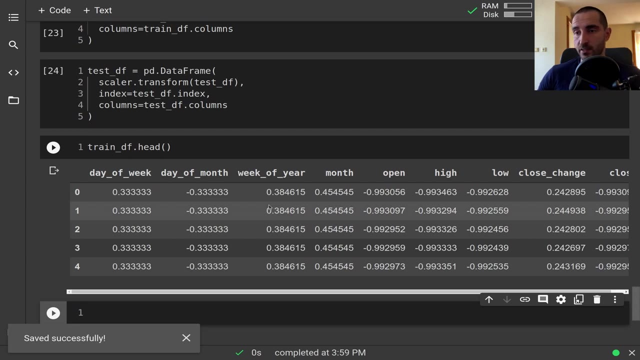 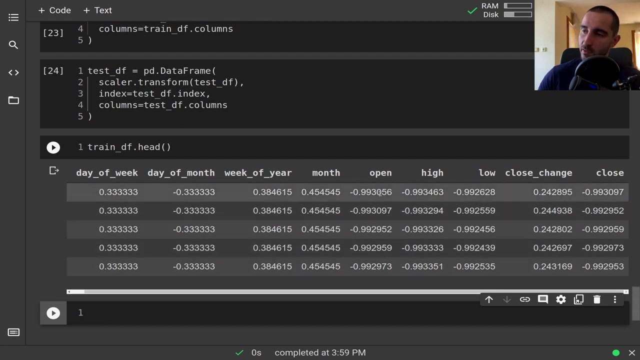 data prime. okay, so run this, and next we let's check what we have into the training data frame now. so basically the same columns, but, as you can see, the numbers are very, very different, at least in the price range. let's compare this with the previous prices we had. 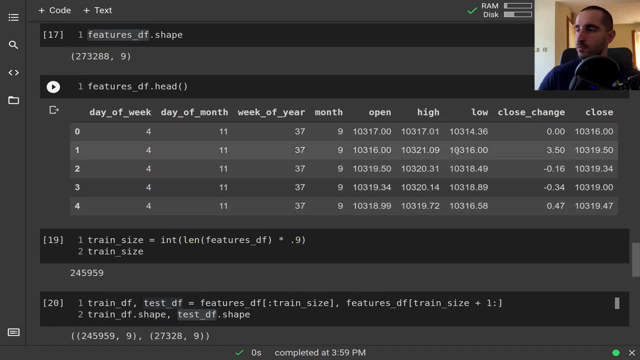 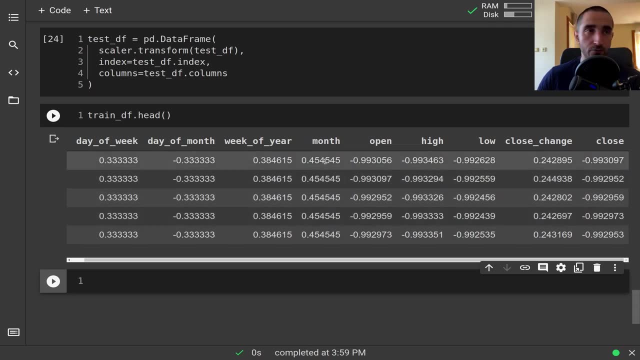 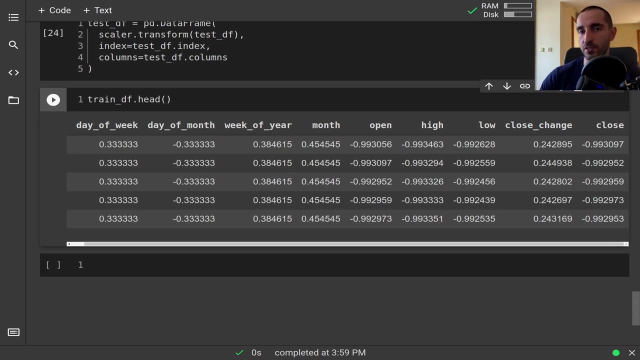 a rather large values- around 10k in us dollars- and now those values are scaled very differently. so this is good. it means that it's doing something at least. and for the final step of the pre-prof sync, we are going to convert those training and test data. 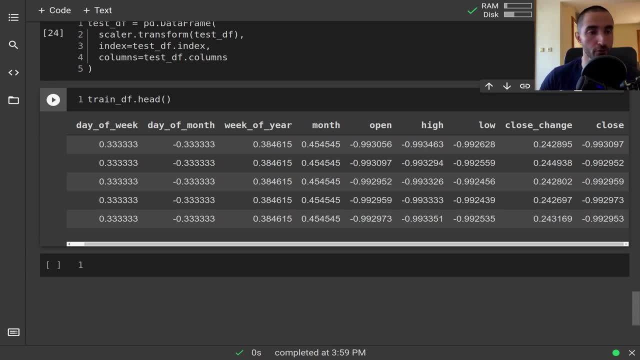 frames into sequences. for that purpose, i'm going to write a new function which we are going to call create sequences, and this function is going to take some input data, which is going to be a pandas date frame. it's going to contain the target column, the column that we want to predict, and the sequence length. 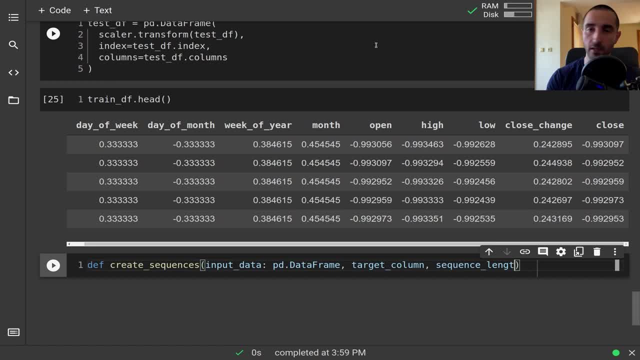 what we are going to do here, then, is basically cut the data into multiple sequences, and i'm going to start by just writing out the function, and then we are going to have a look at an example of how it's going to work. so please stay with me. so the sequences are going to be a list. 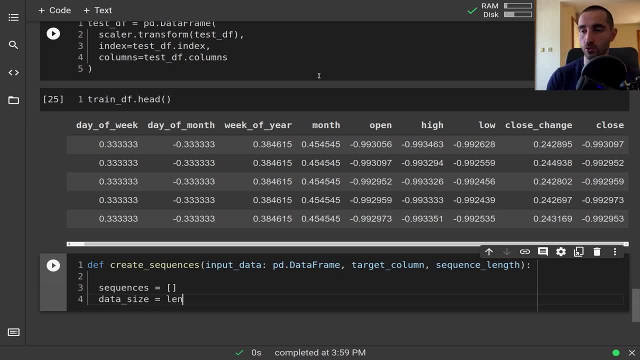 right here, and then we are going to check the number of rows into the input data. next, we are going to iterate over the data, and we are going to again use tqdm, and i'm going to iterate over the range of data size minus the sequence length. so what will this do is iterate over all of the data, except for the last examples, which are going. 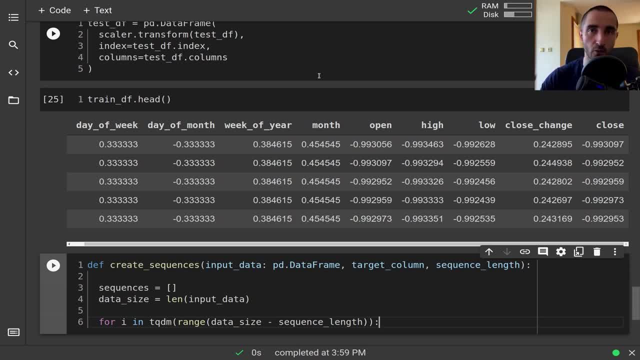 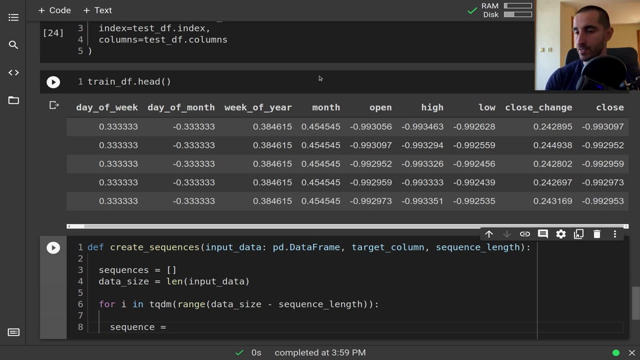 to be the number of sequences that we have, and this is required because otherwise we are not going to have enough at the end to basically go through the sequences. so the first thing that i'm going to do is get the sequence and i'm going to use the input data. 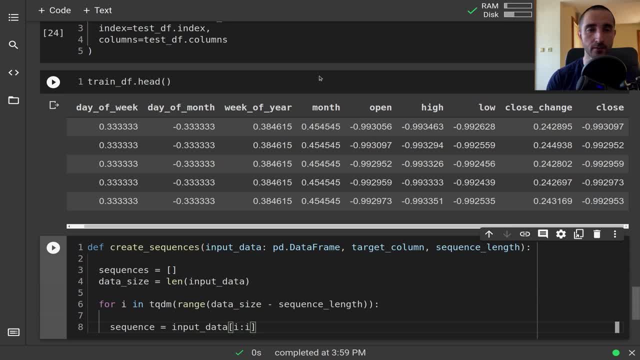 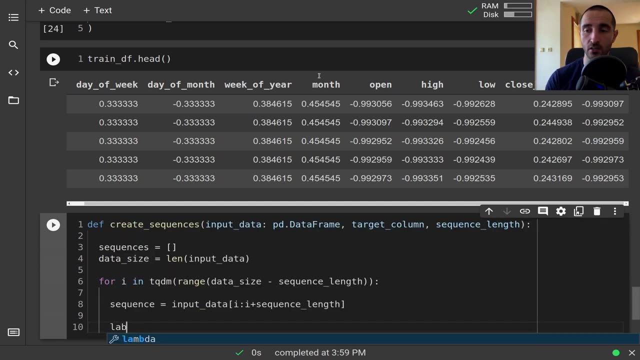 from ith index to i plus sequence length. so this will give us a sequence with the length of the past parameter that we have, and next i'm going to take the next value, which is going to be the position of the label, and this is going to be i plus sequence length, and this is exclusive, so we 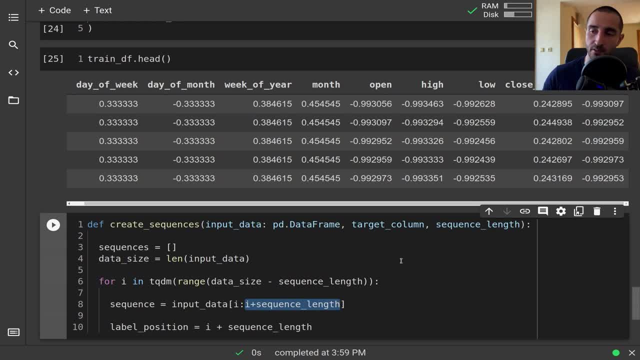 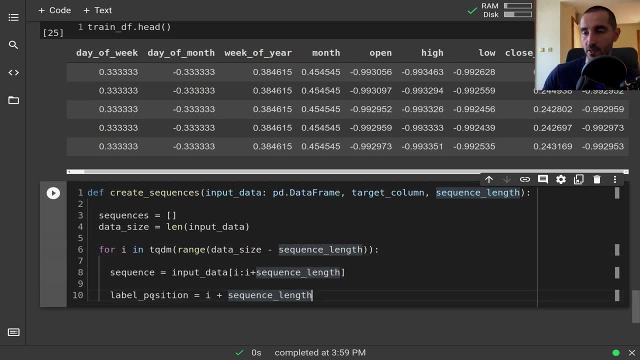 are not getting uh this, but we are getting this minus one. so this is basically how the indexing in python works. so the label position right here is going to be integrated in this. so label position position right here is going to be at this position, which is inclusive. i know this might. 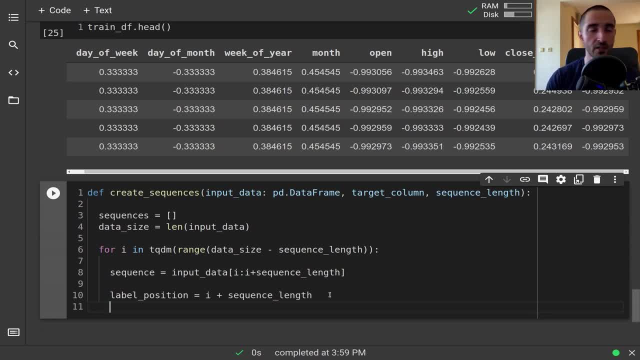 be a bit of hard to get at first, but i hope that when we look at the examples this all makes sense. next i'm going to take the label value itself and i'm going to take the label position role and from that i'm going to take the target column. so this will just give us the role value that we 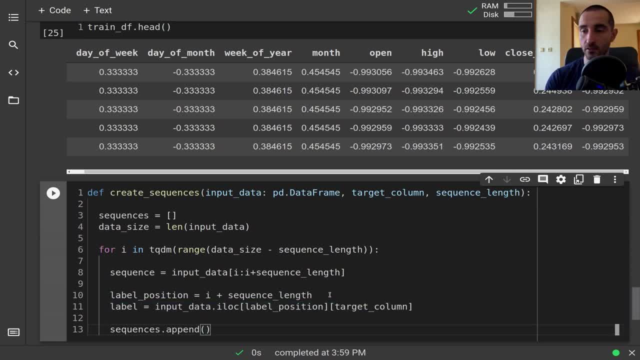 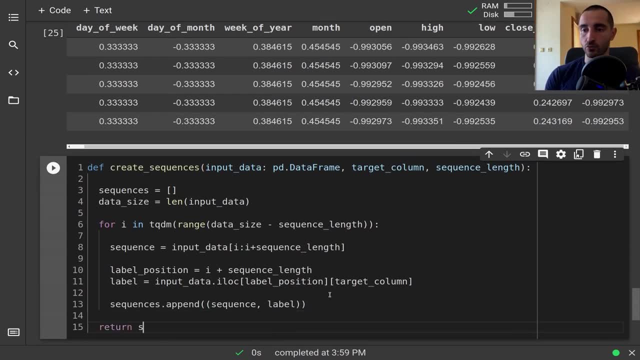 have, and next i'm going to append the sequence, or a tuple of the sequence, and the label. finally, i'm going to return the sequences, and this is pretty much the function that we need. of course, you might go ahead and try something a bit more advanced, like, for example, sliding windows or maybe another variation of that. 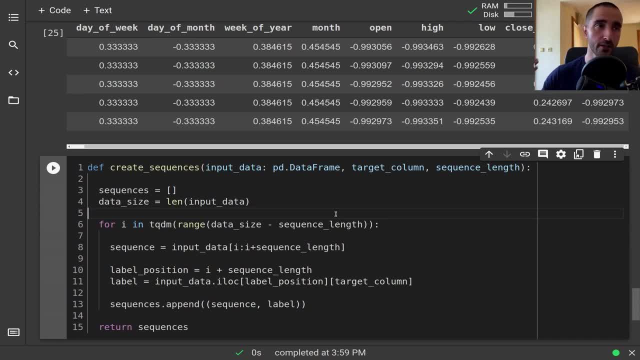 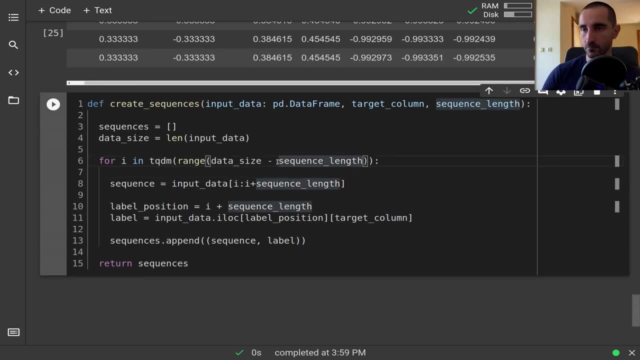 this is a really simple implementation in which we are taking every next value and just creating a sequence out of it. so let me run this- and i have a little example of here, right here, and i'm going to create a dummy, and i'm going to create a dummy. 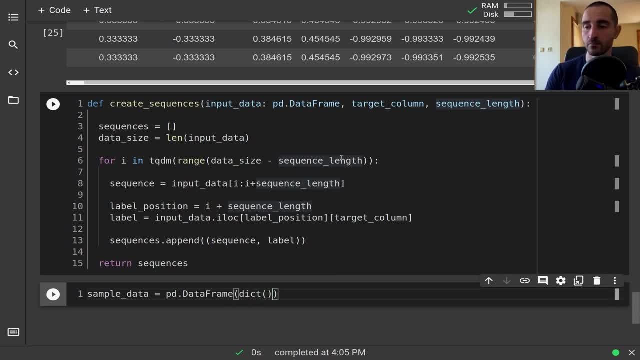 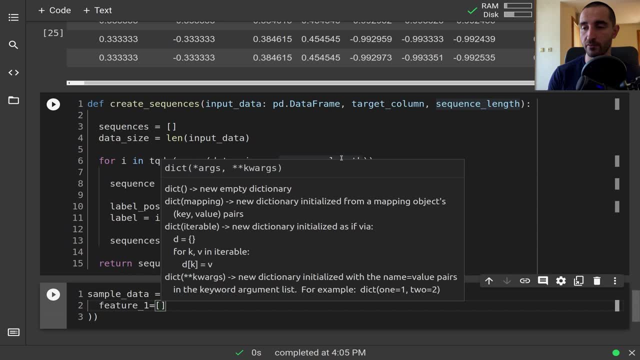 and i'm going to create a dummy data frame, and here i want to create a feature, and here i want to create a feature, and here i want to create a feature which will have the values, which will have the values, which will have the values, yeah, yeah. 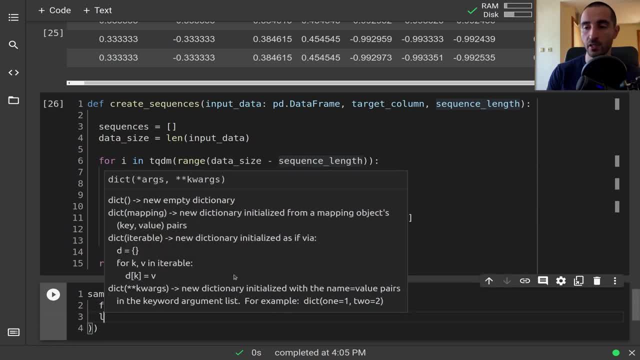 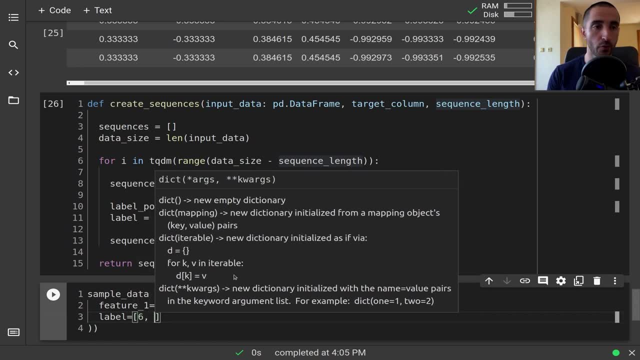 yeah, one, two, three, four and five. one, two, three, four and five. one, two, three, four and five, and i have, uh, i'll have a column with the name of label, with the name of label, with the name of label: six, seven, eight, six, seven, eight, six, seven, eight, nine, ten. 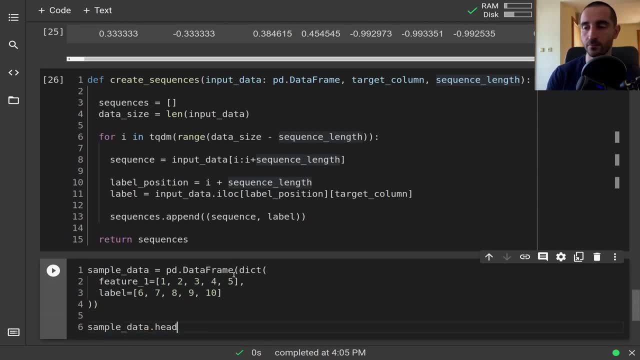 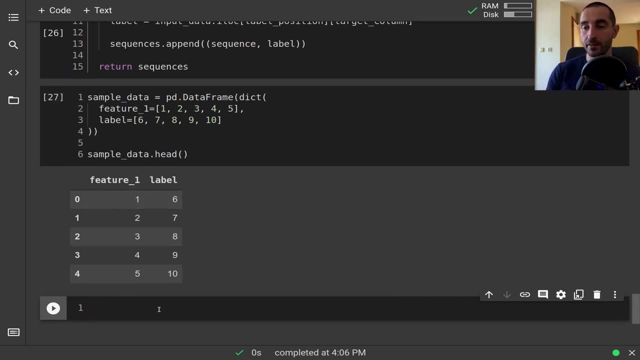 nine, ten, nine, ten. let's look at the data. let's look at the data. let's look at the data right here. okay, so we have this very basic data frame. okay, so we have this very basic data frame. okay, so we have this very basic data frame and let's create sequences. 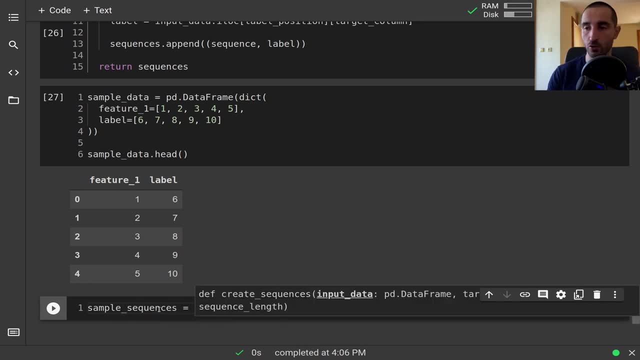 and let's create sequences, and let's create sequences from this. we'll call, we'll call, we'll call the function create sequences. we are the function create sequences. we are the function create sequences. we are going to pass in the label as target. going to pass in the label as target. 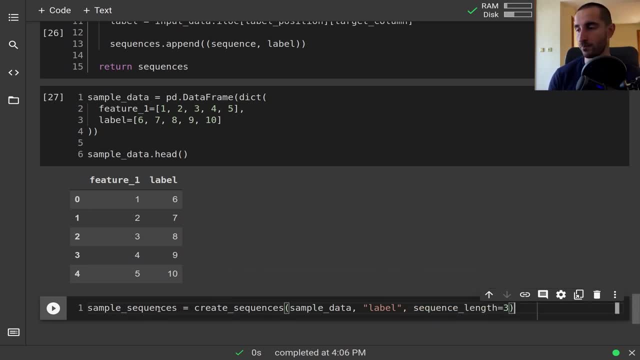 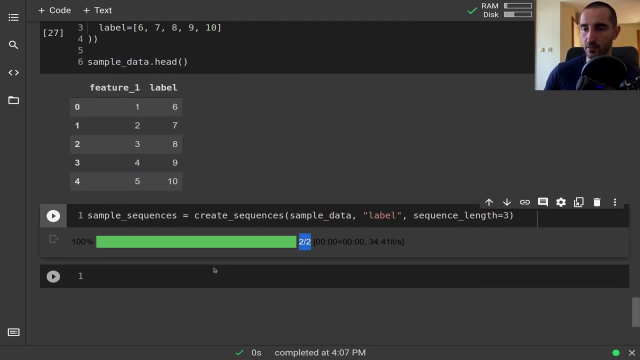 going to pass in the label as target variable and the sequence length is variable, and the sequence length is variable, and the sequence length is going to be three, going to be three, going to be three. let's say, let's say, let's say so. so, so this runs and it's already telling us. 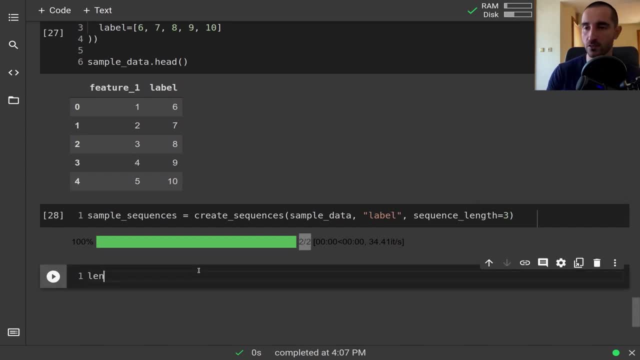 this runs, and it's already telling us this runs, and it's already telling us that it did that, it did that, it did two iterations, two iterations, two iterations. so the number of, so the number of, so, the number of sequences should be two. sequences should be two. 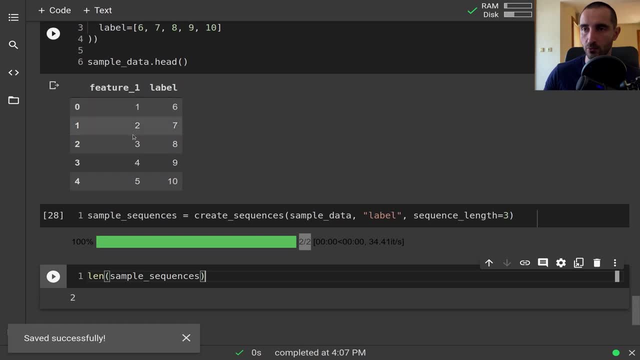 sequences should be: two and you might, and you might, and you might think that one, two, three, think that one, two, three, think that one, two, three, two, three, four, two, three, four, two, three, four and three four, five are the possible, and three four, five are the possible. 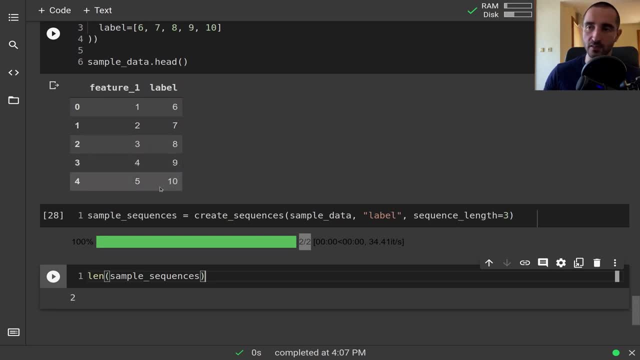 and three, four, five are the possible sequences that you can get, sequences that you can get, sequences that you can get, but that's not exactly correct because. but that's not exactly correct because. but that's not exactly correct because for the was sequence, you basically. for the was sequence, you basically. 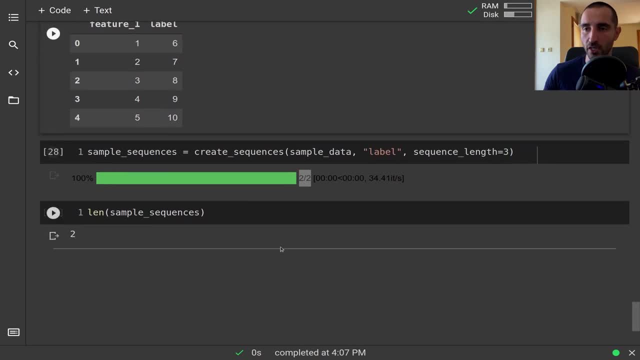 for the was sequence. you basically don't have a label, don't have a label, don't have a label. so let's check, so, let's check, so let's check the la, the sequences themselves, the la, the sequences themselves, the la, the sequences themselves. and to do that, i'm going to 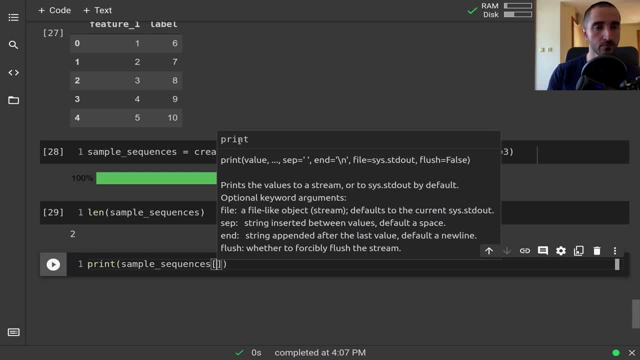 and to do that i'm going to, and to do that, i'm going to first take the sequence first. take the sequence first. take the sequence at zero position, at zero position, at zero position. this will give us the sequence, then i'm. this will give us the sequence, then i'm. 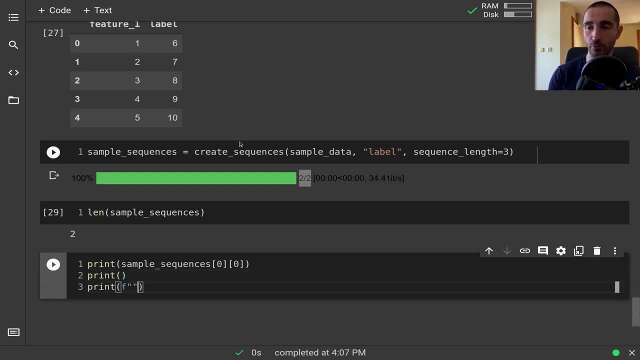 this will give us the sequence: then i'm going to print out a row, going to print out a row, going to print out a row, and then i'm going to print out the, and then i'm going to print out the, and then i'm going to print out the label. 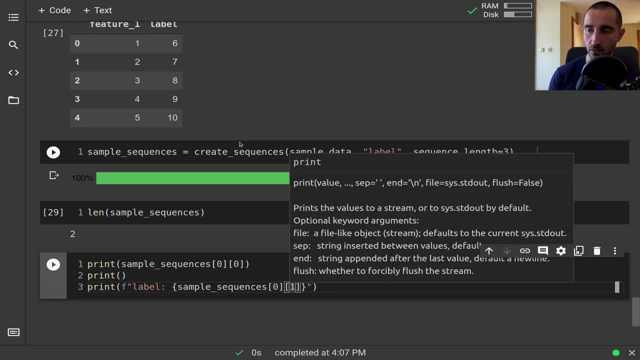 at the zeroed position, so the first at the zeroed position, so the first at the zeroed position. so the first, sequence, sequence, sequence. the label itself and the label itself and the label itself, and this gives us the first three. this gives us the first three. 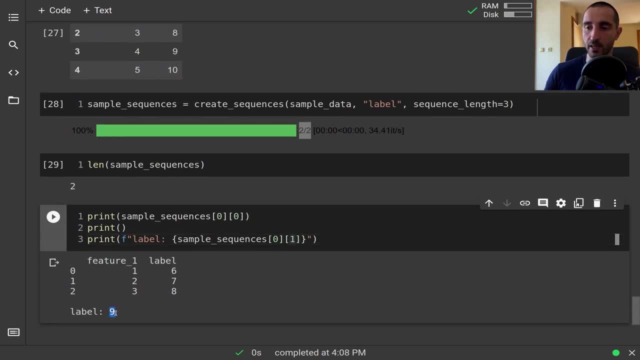 this gives us the first three rows from the: the data frame. rows from the: the data frame rows from the: the data frame. and then the label is the next, and then the label is the next, and then the label is the next. the label from the next. the label from the next. 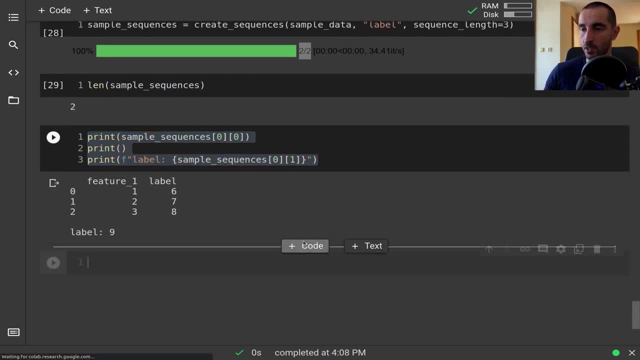 the label from the next row. so this works as expected row. so this works as expected row, so this works as expected, and then, and then, and then we have the next example which is going, we have the next example which is going, we have the next example which is going to be the next sequence. 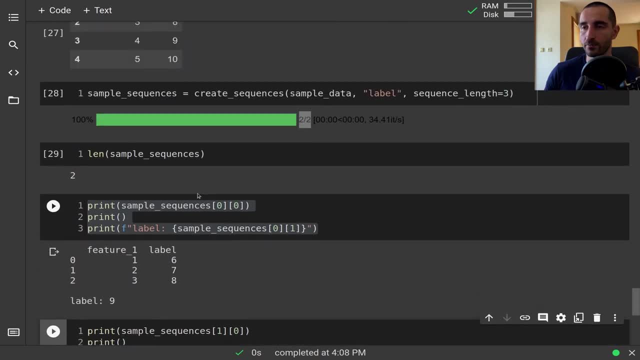 to be the next sequence, to be the next sequence, and for this one we have two, three, four, and for this one we have two, three, four, and for this one we have two, three, four, two, three, four, seven, eight, nine. two, three, four, seven, eight, nine, two, three, four, seven, eight, nine and the label is ten. 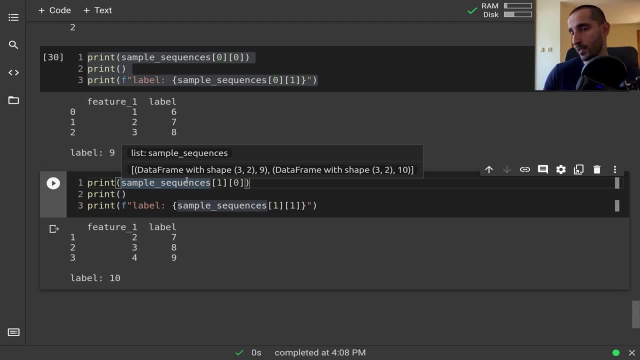 and the label is ten. and the label is ten, so note that we don't have any more. uh, so note that we don't have any more. uh, so note that we don't have any more. uh, we don't have any more labels. so this is. we don't have any more labels, so this is. 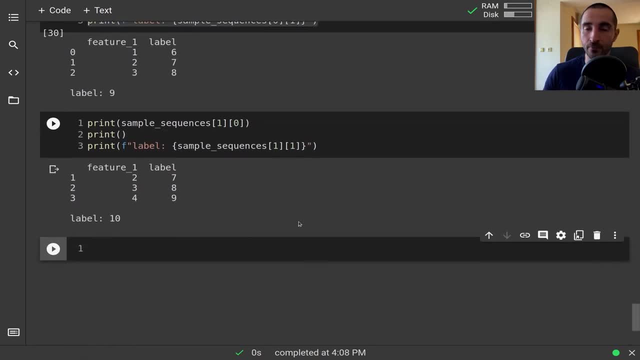 we don't have any more labels. so this is why the number of sequences is two, why the number of sequences is two, why the number of sequences is two. all right, all right, all right. i hope that all this makes sense. and i hope that all this makes sense and 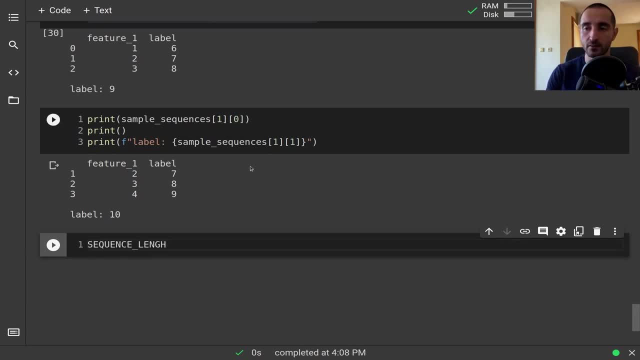 i hope that all this makes sense. and next i'm going to create a sequence. next i'm going to create a sequence. next i'm going to create a sequence. length: constant, constant, constant. i'm going to pass in, for example, 60. i'm going to pass in, for example, 60. 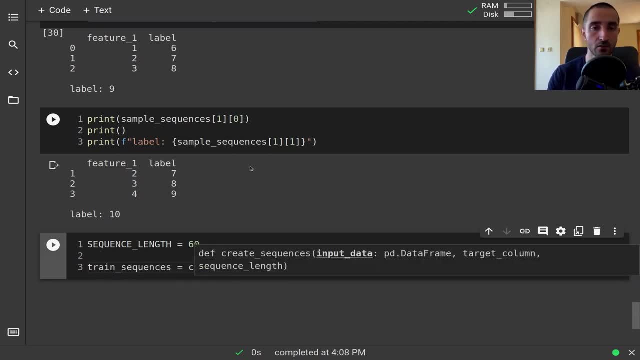 i'm going to pass in, for example, 60, i'm going to create a training, i'm going to create a training, i'm going to create a training, sequences, sequences, sequences, using the training data frame, and i'm going to pass in the sequence and i'm going to pass in the sequence. 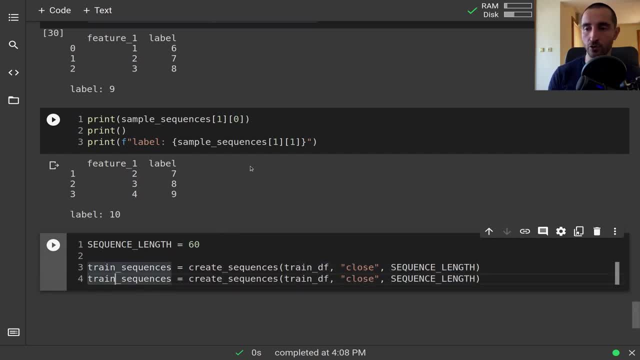 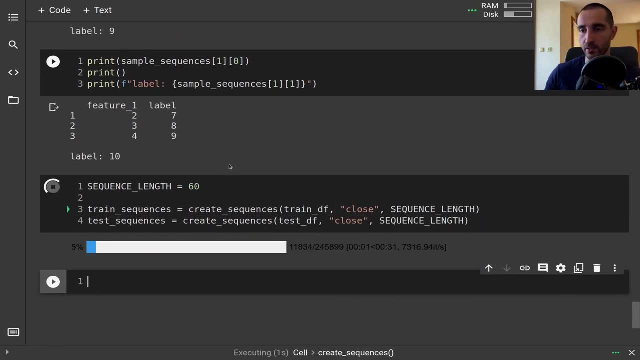 and i'm going to pass in the sequence length. i'm going to do the same thing. i'm going to do the same thing. i'm going to do the same thing for the, for the, for the best sequences and basically best sequences and basically best sequences, and basically related run. 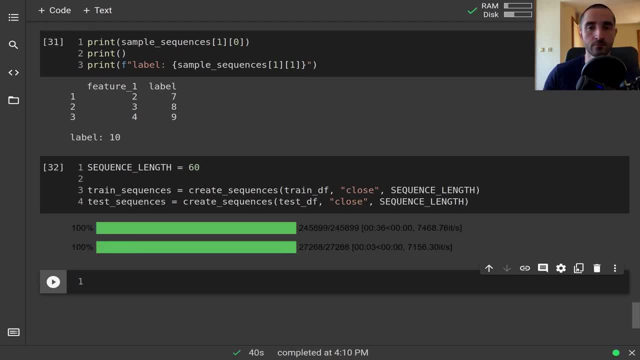 related run: related run: now that the pre-processing is complete, now that the pre-processing is complete. now that the pre-processing is complete, it roughly took about 40 seconds. it roughly took about 40 seconds. it roughly took about 40 seconds combined, combined. combined. here is the output of that. 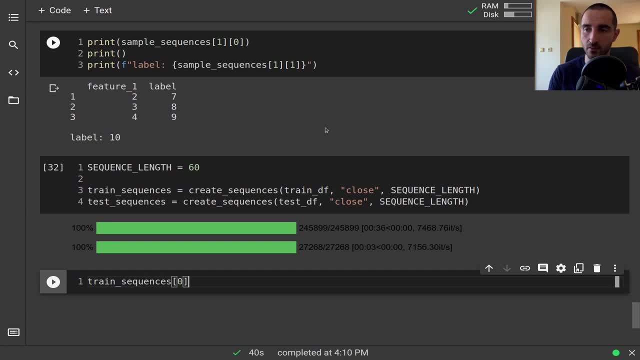 here is the output of that, here is the output of that. and let's check, for example, the first. and let's check, for example, the first. and let's check, for example, the first sequence, sequence, sequence. what does it have? let's first check the. what does it have? let's first check the. 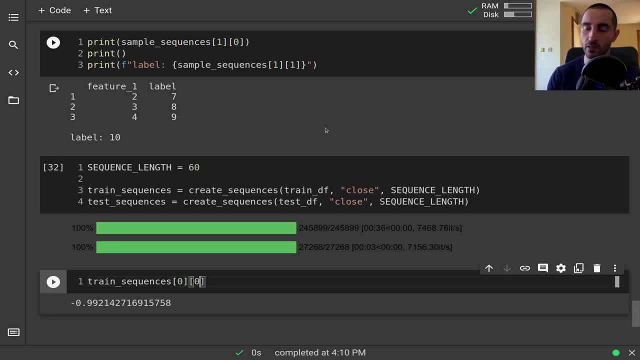 what does it have? let's first check the label: label, label. so this is just the number and the so. this is just the number and the so this is just the number and the sequence. sequence, sequence is going to be, is going to be, is going to be basically this: 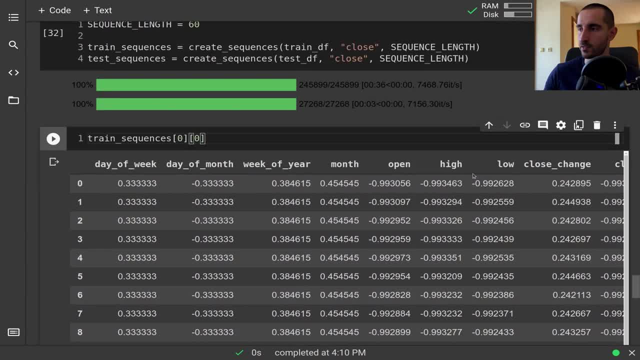 basically this, basically this. i believe that this is a data frame. i believe that this is a data frame. i believe that this is a data frame. actually, yeah, it's a date frame which actually, yeah, it's a date frame which actually, yeah, it's a date frame which contains all the 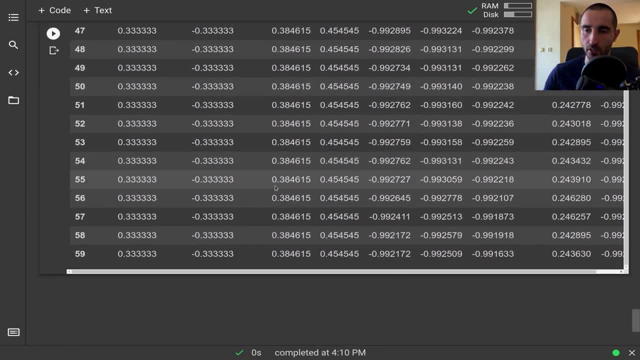 contains all the contains all the examples, examples, examples that we want, that we want, that we want, and this should be 59 because it starts, and this should be 59 because it starts, and this should be 59 because it starts from, from from zero. so we have. 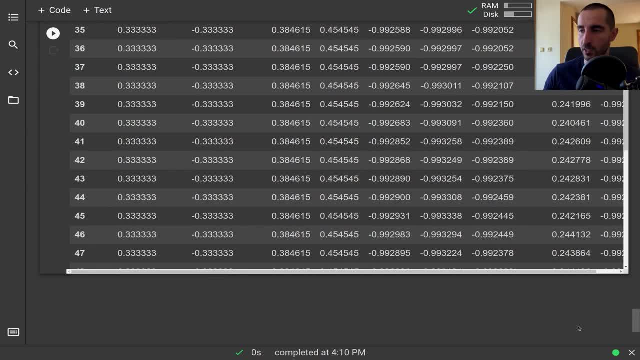 zero, so we have zero, so we have a data frame that contains 60 rows, a data frame that contains 60 rows, a data frame that contains 60 rows, and this will be, and this will be, and this will be a sequence that is created. a sequence that is created. 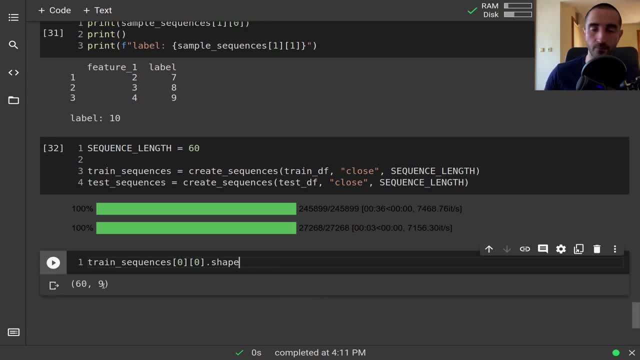 a sequence that is created from the large training data frame, this from the large training data frame, this from the large training data frame. this is the shape of it and to basically is the shape of it and to basically is the shape of it and to basically check how many sequences that we have. 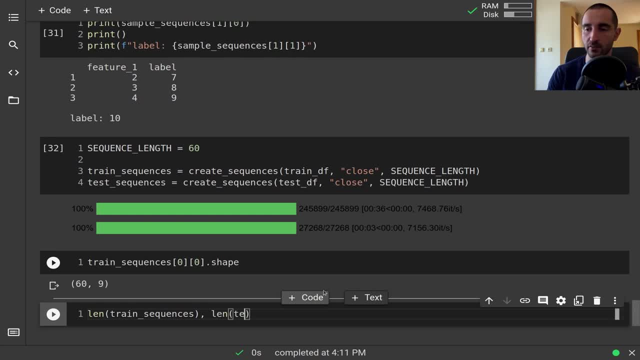 check how many sequences that we have, check how many sequences that we have. have the training sequences, have the training sequences, have the training sequences and the length of the test and the length of the test and the length of the test. sequences right here. sequences right here. sequences right here. so 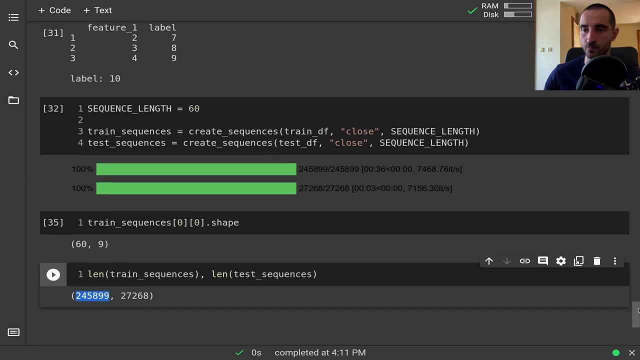 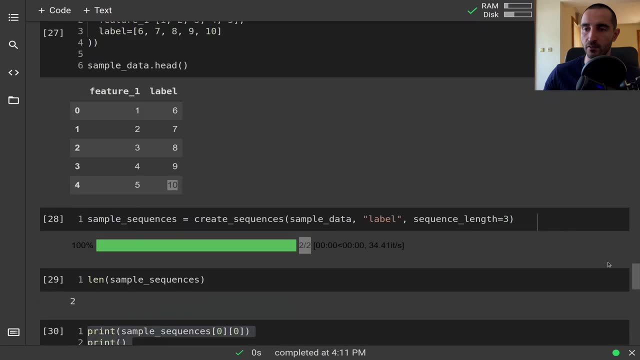 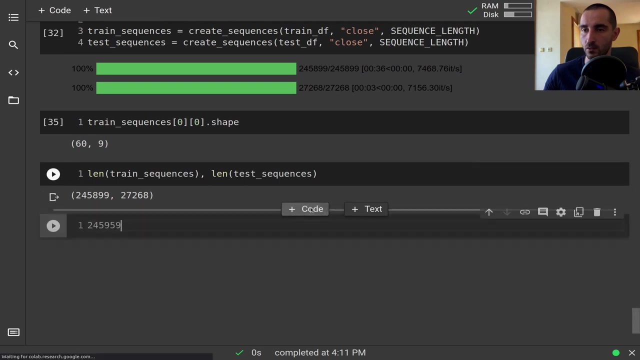 so, so this is, this is, this is: let's compare this to the, let's compare this to the, let's compare this to the, to the training data frame. so, as you can see, let me just copy this, let me just copy this, let me just copy this. 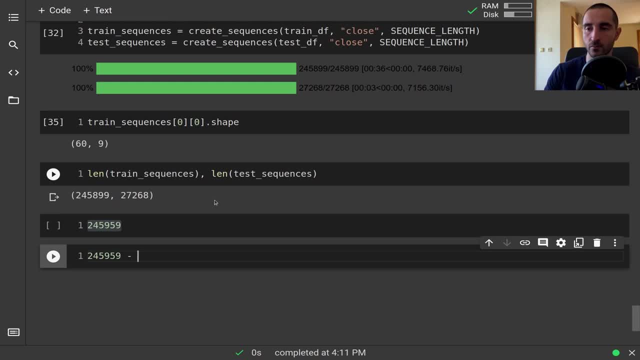 this is the number of examples that we get into the training examples that we get into the training examples that we get into the training data frame. and if we do this data frame, and if we do this data frame, and if we do this, you can see that this is exactly. 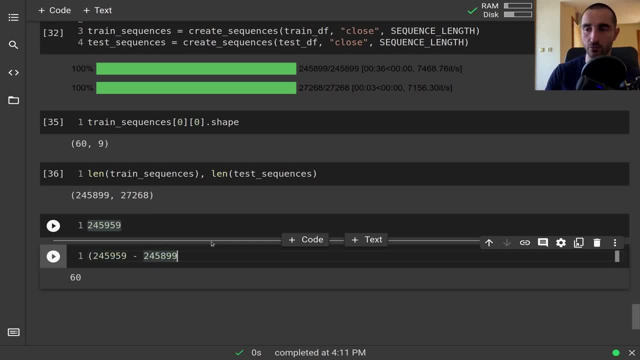 you can see that this is exactly. you can see that this is exactly the, the, the. so this should be, so, this should be, so this should be true, true, true. if we did everything correctly, if we did everything correctly, if we did everything correctly, so this should be exactly. 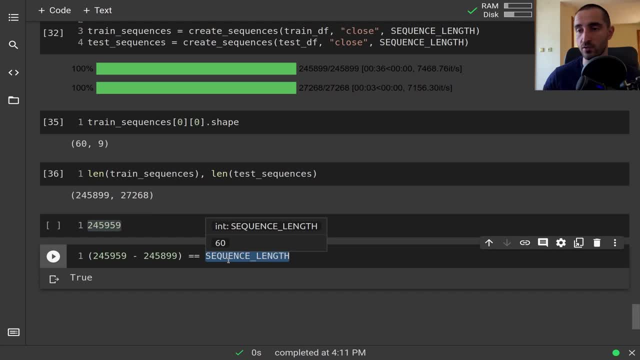 so this should be exactly, so this should be exactly the number of the elements that we have, the number of the elements that we have, the number of the elements that we have into each sequence, into each sequence, into each sequence. so everything, so, everything, so everything kind of. 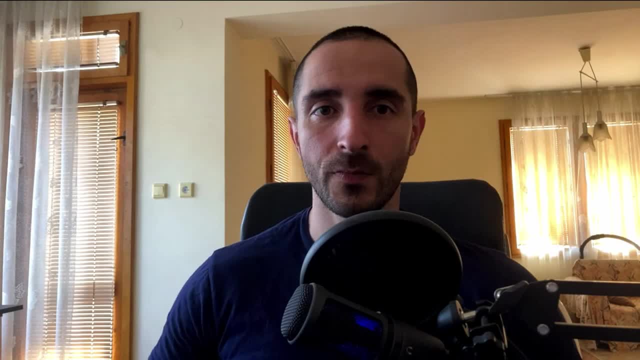 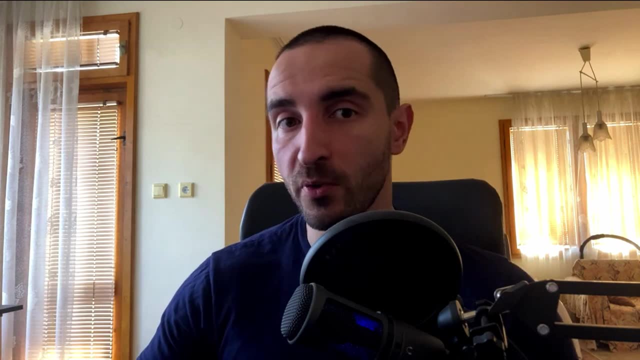 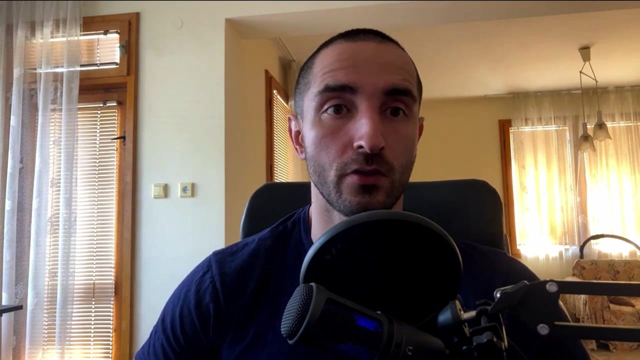 checks out. so this is great and- and this is pretty much how you can pre-process your time series data. again, we had multiple features. you can do the same thing basically for a single feature. there is no reason that why this shouldn't work. you might need to do some fiddling, but it should.